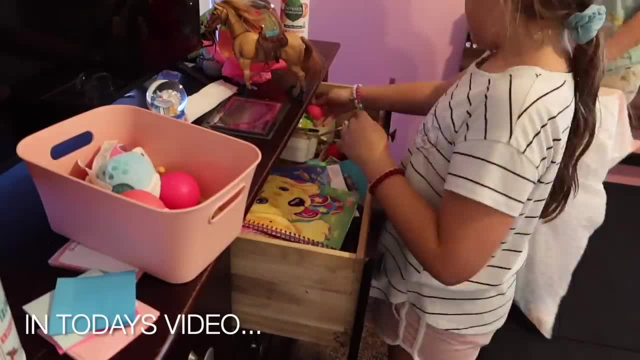 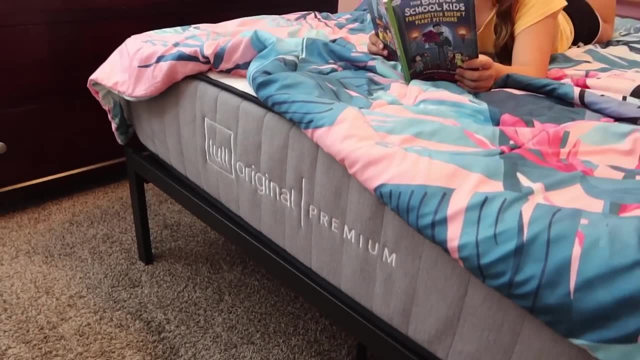 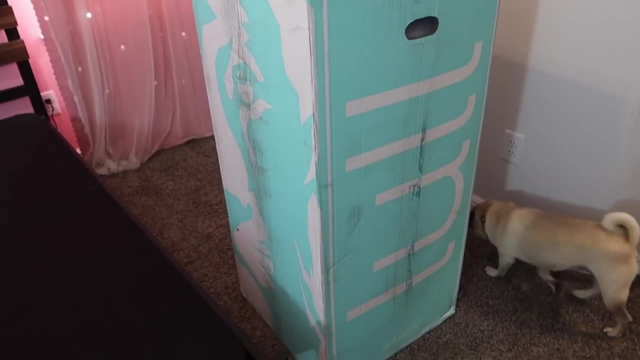 the transformation first, and then you'll see the process of me doing it. And that is because today's video is sponsored by Lull. So thank you so much, Lull Mattress for sponsoring today's video. We were beyond excited to receive this mattress, which is their original premium mattress. We have it in the size full. 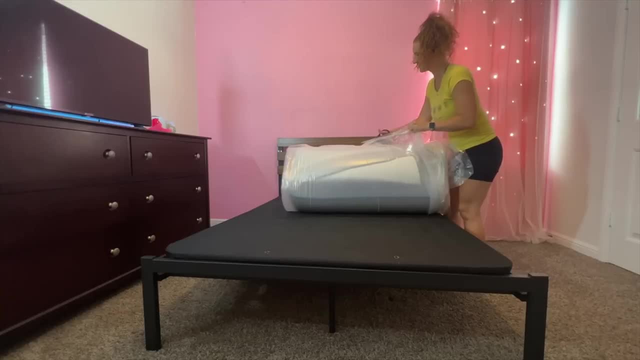 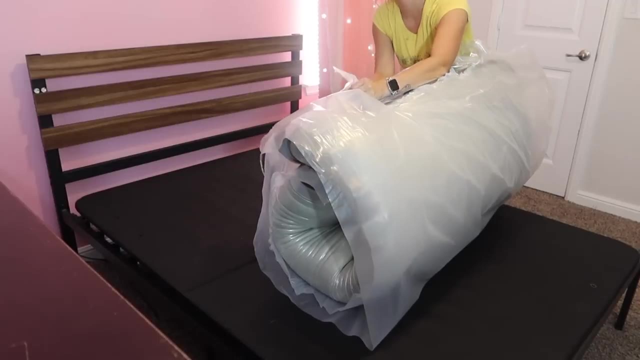 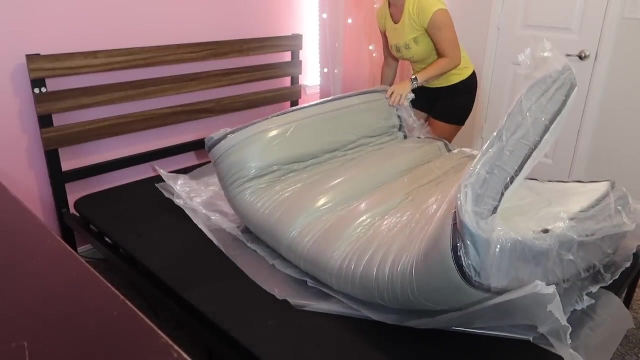 and it is made out of 100% premium memory foam. It adapts perfectly to your body's unique shape to provide rest and rejuvenation. It also has cooling gel infused beads paired with open cell memory foam which works together to redirect the heat away from your body. So you get a good 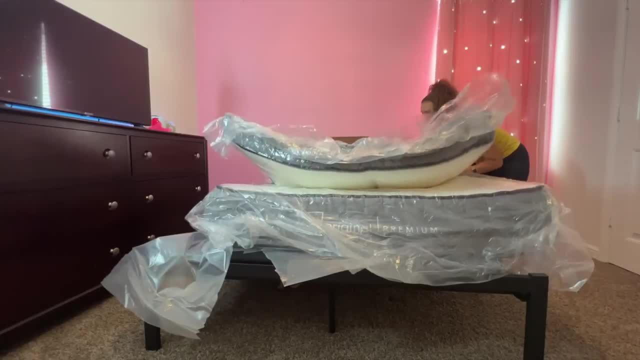 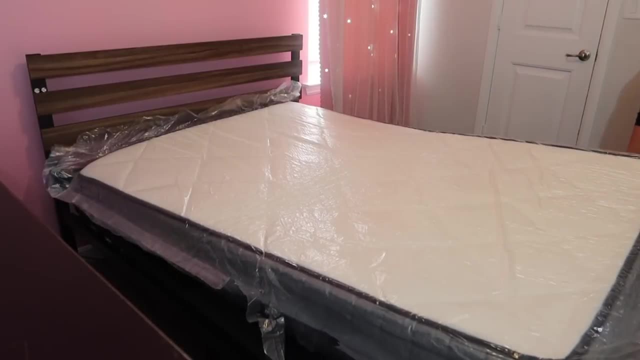 night's sleep. And another great feature is that you do not need a box spring, which is a great feature for your mattress. It is a 12 inch long and of the highest quality foam. That way, you have the right firmness and support. but it's also a standalone mattress And since 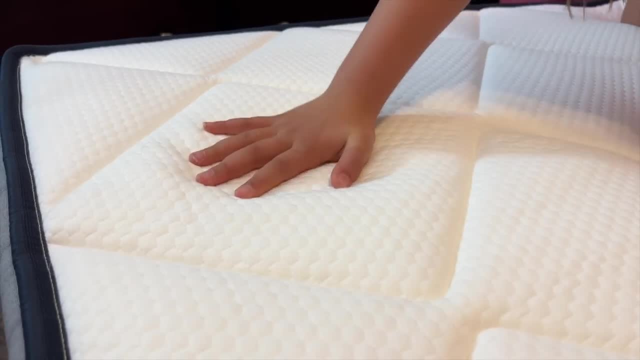 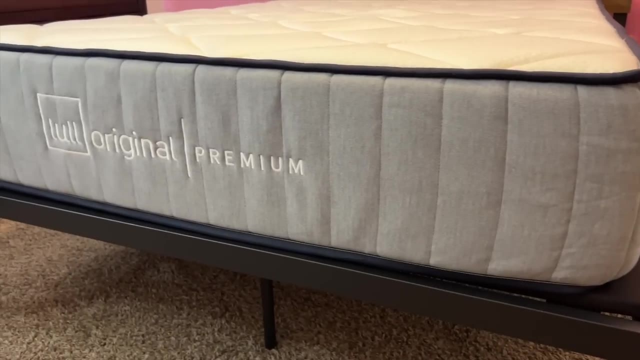 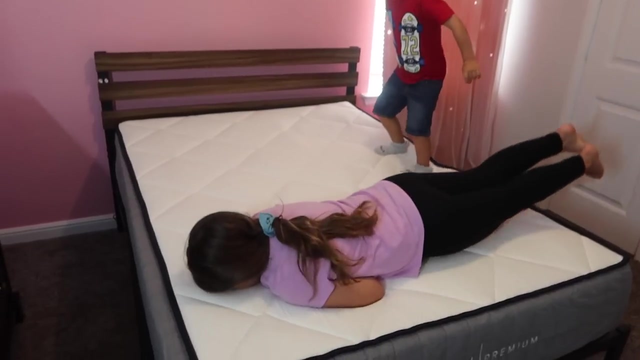 Adrienne has gotten her new mattress. she has said nothing but amazing things about it. In her own words, she said it's the best mattress she has ever had, And I can attest to that, because she's sleeping in even later now And both me and my husband tried it out and we loved it And we're 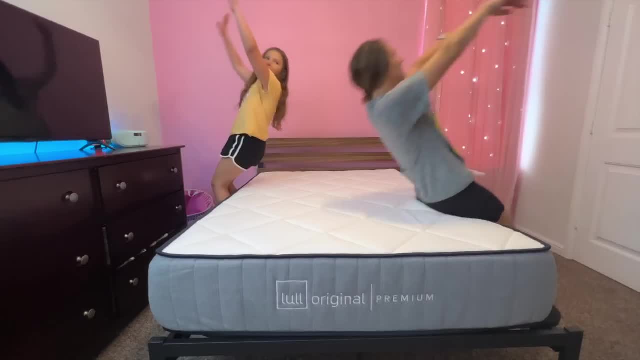 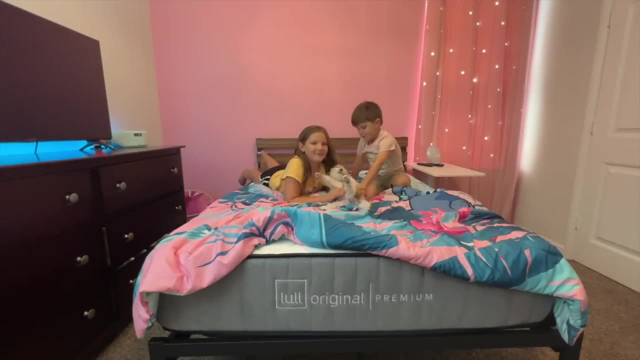 love this mattress as well. It's the perfect amount of firmness, but it's really soft. Both me and my husband like a softer mattress, and this is definitely a softer mattress, but still gives you the support that you need to get a good night's sleep. I definitely recommend this You. 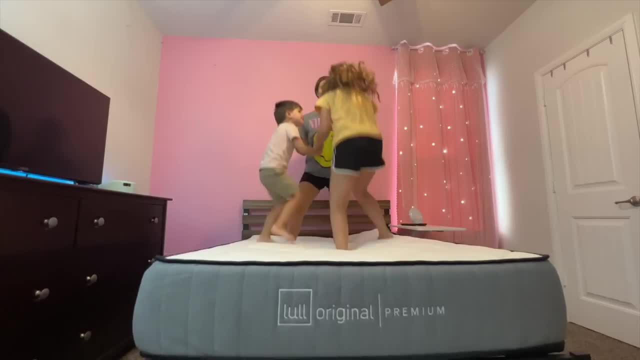 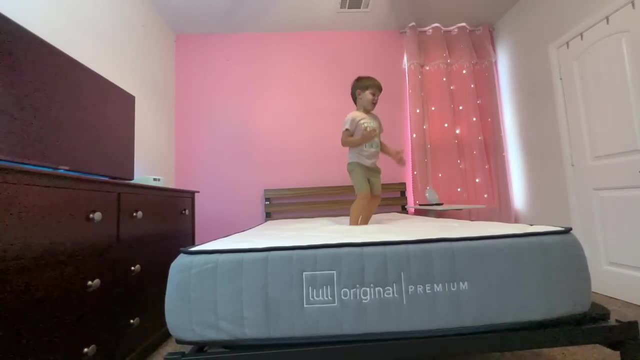 guys. it is so comfortable. So if you guys are in the market and looking for a new mattress, make sure y'all use my link down in the description. It will save you up to $700 off of your mattress And I can assure you that it's going to be a great mattress for you. 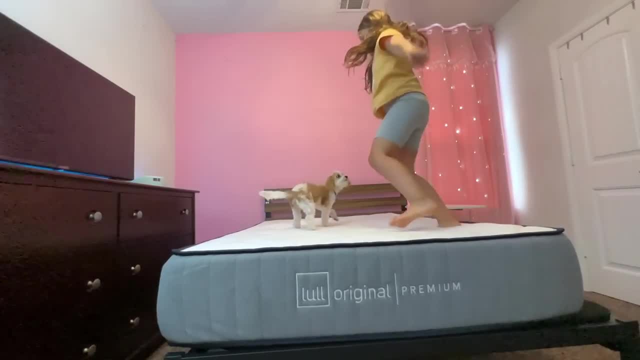 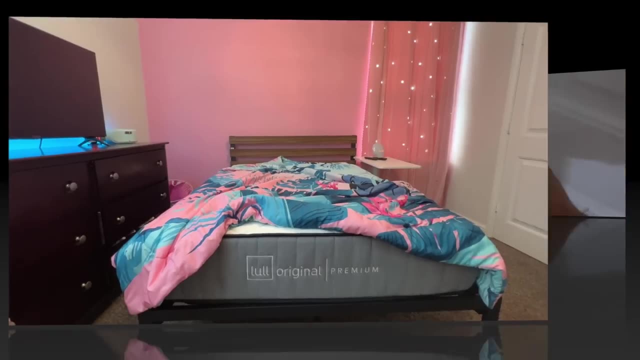 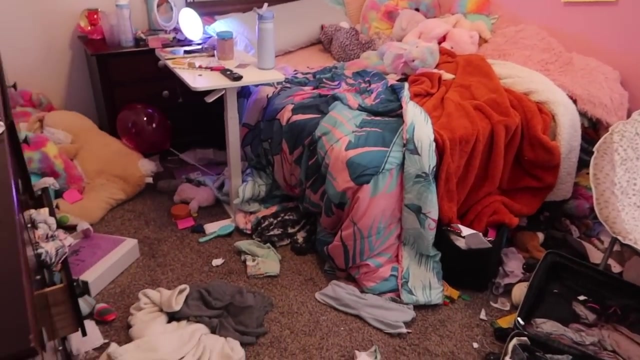 You guys are going to love it. So, once again, thank you so much, Lowell, for sponsoring today's video. but now it's time to get into all of this decluttering and organizing and cleaning motivation, And let me tell you, it is going to be a super satisfying one. Her room is trashed. 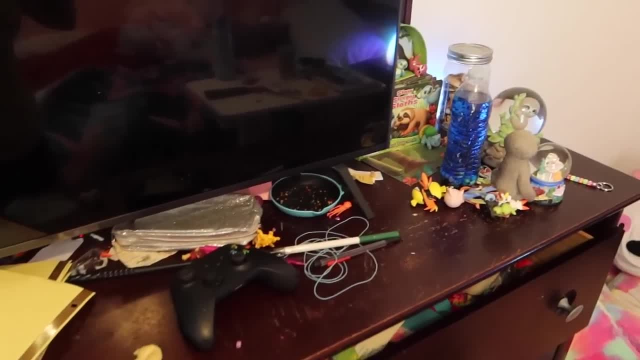 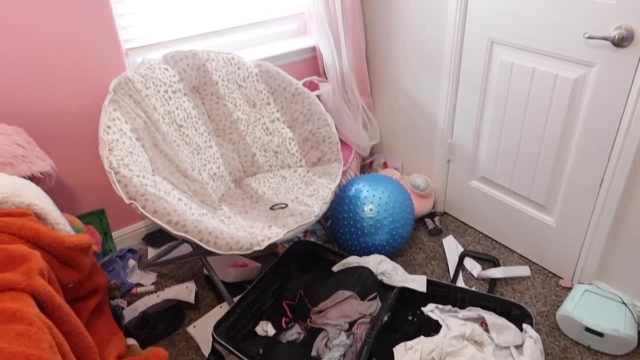 like usual. no surprise there. So the goal was to, of course, get rid of all the trash and clutter, but also rearrange her furniture, just because the room was feeling a bit tight cluttered. We have way too much furniture in here, So I told her it's. 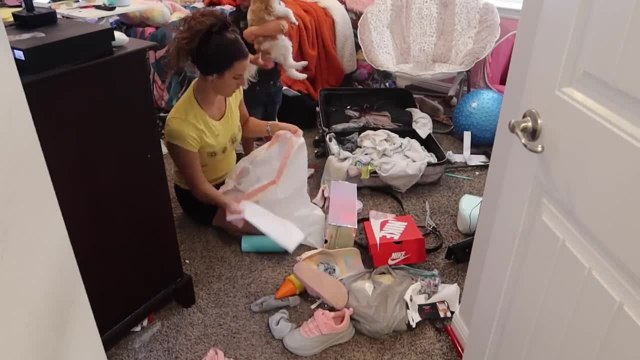 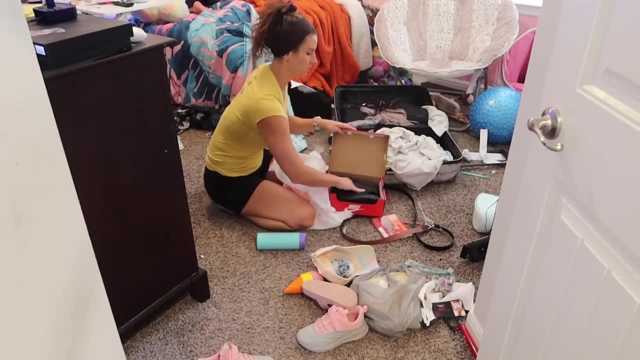 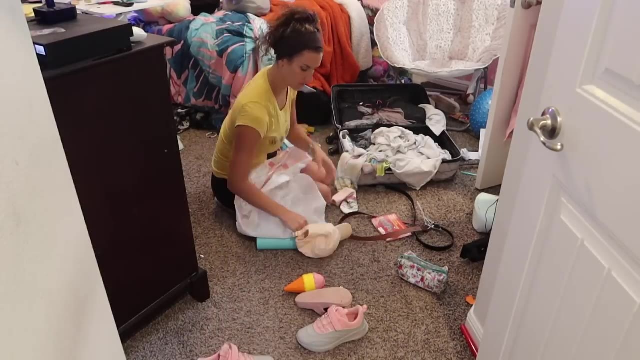 time to not only part ways with some stuffed animals, but also with her nightstand, because most of the things that were in her nightstand could fit in the little cubbies that we have inside of her closet. So that was on my to-do list. I was going to take everything out of her. 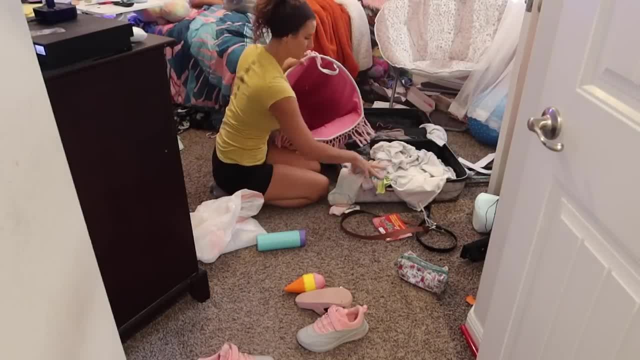 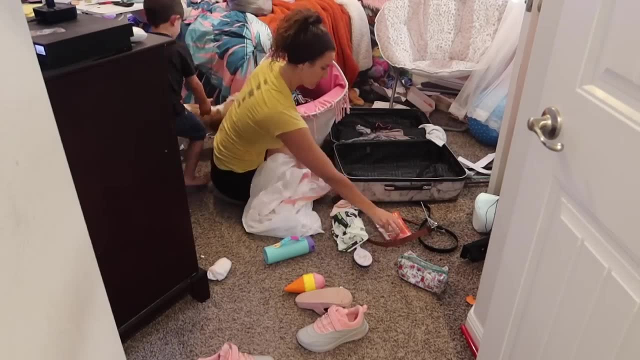 nightstand, go through it, move it into her closet. And, of course, Adrienne will also be me most of the time Whenever I do her room declutter. she's typically at school, but you guys know it's summer break. Well, at least for a little bit longer. they are about to start school. 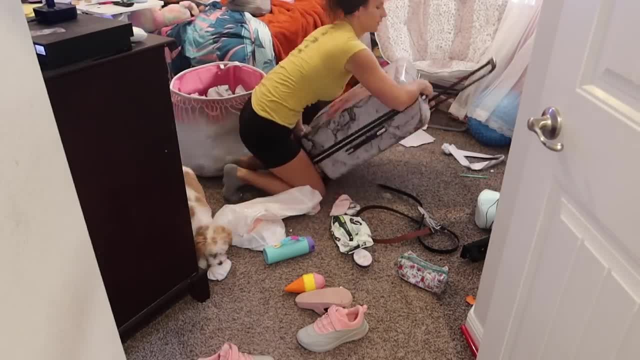 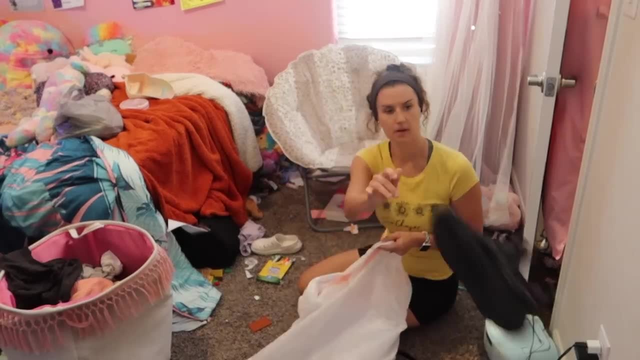 But since she was home, I was like you know what, I'm going to have her go through her things because I'm a bit more conservative. I'm not sure like what she plays with what she doesn't, So I don't want to throw away things that I'm not sure if she still uses. So I typically hold on. 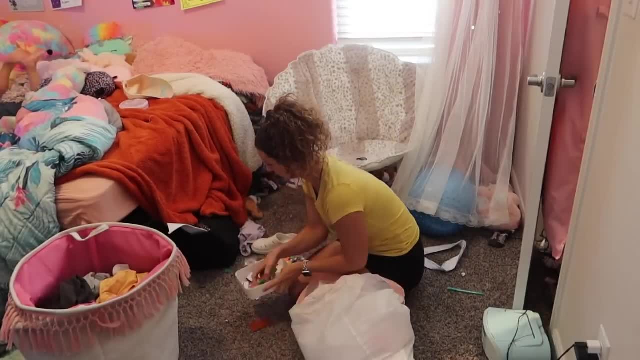 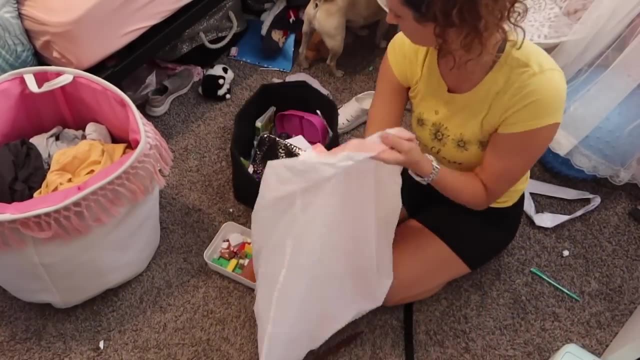 to quite a bit of things. And then you know I'm going to have her go through her things. We end up here again where stuff is just everywhere and super cluttered. So I knew I wanted her to go through her things, get rid of a lot. And let me tell you I was so proud of her. 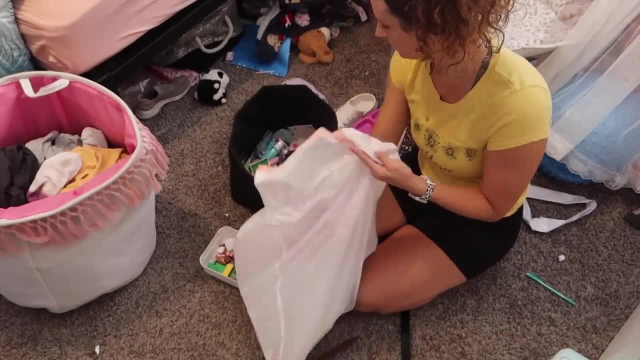 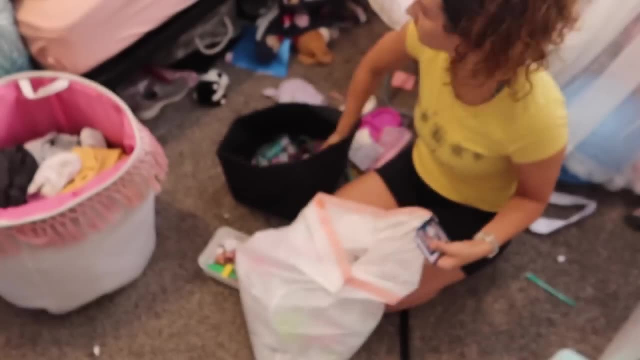 She definitely is a sentimental person. Like you know, things hold a lot of value to her and a lot of memories, which is understandable because I feel like a lot of us are like that, but she did really good and got rid of a lot of stuff. 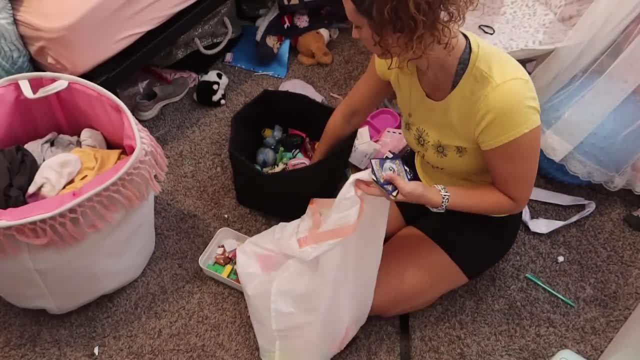 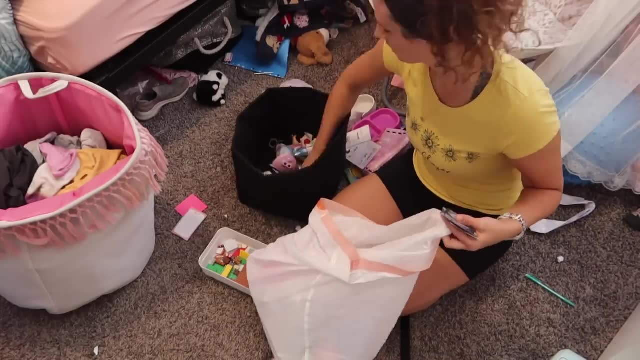 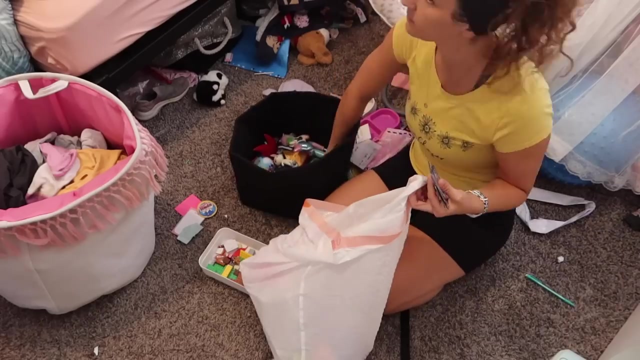 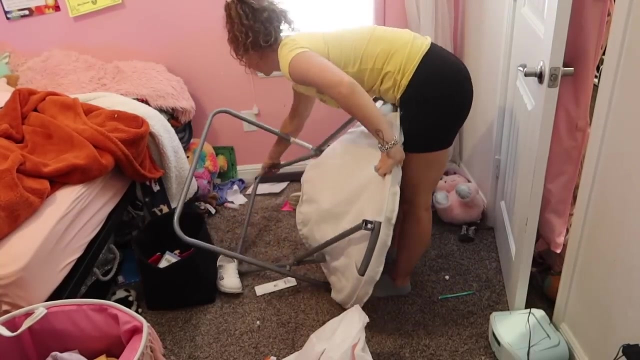 So we have a few bins that typically are stored underneath her bed that hold a lot of her toys. She's not like a huge toy person, She has a few like little odds and ends, mainly fidgets and stuff like that. So everything that she plays with is pretty small. So they're either in her 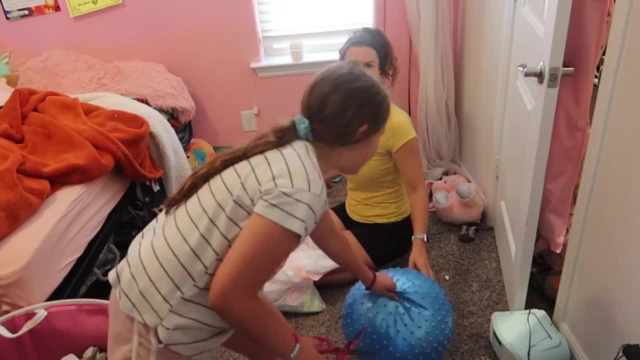 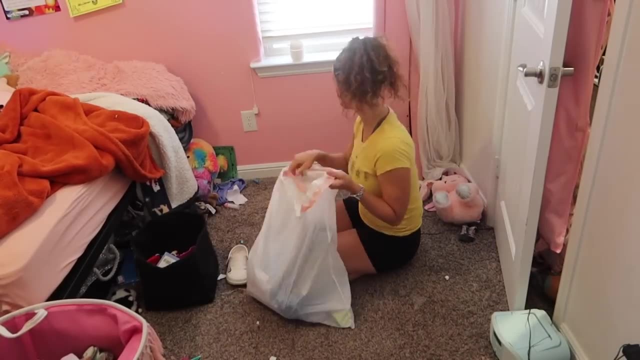 trunk or in her closet, So she's not like a huge toy person. She has a few like little odds and ends or the few little baskets that are under her bed. So I was just going through her basket and getting the trash out, because she's very creative and she's always making things with 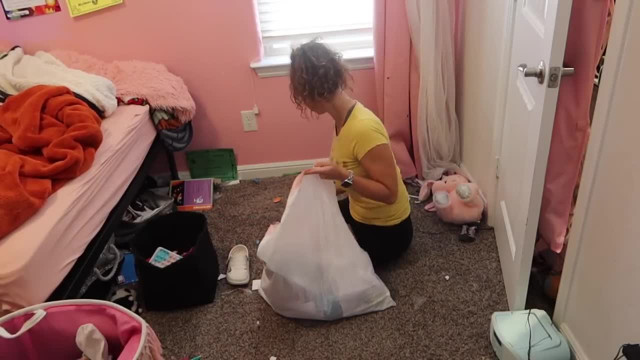 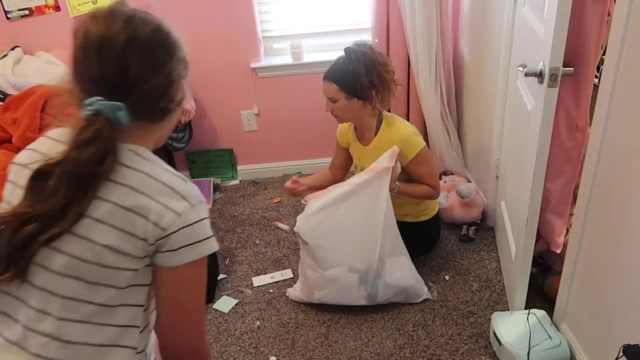 paper and beads and string And the trash was insane in here, You guys. I mean majority of what I got rid of was just paper, So I wanted to first go through it, get the trash out of it, And then I was going to have her go through the actual toys. 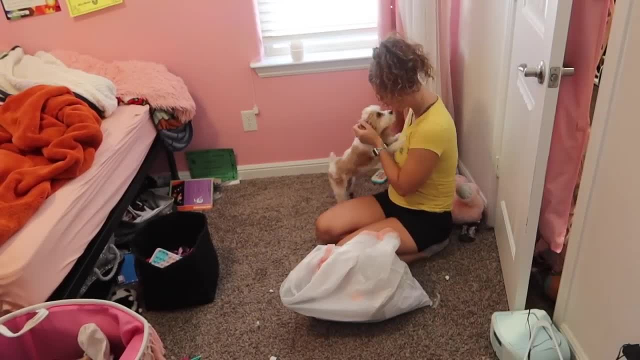 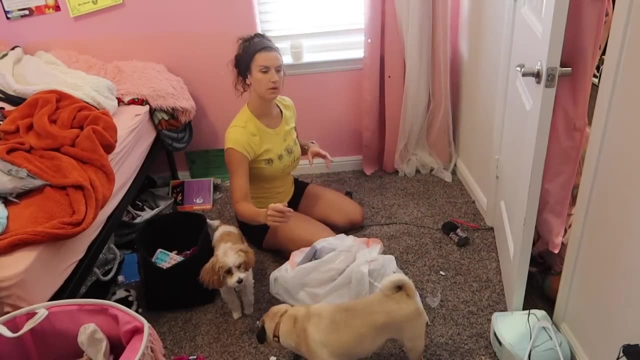 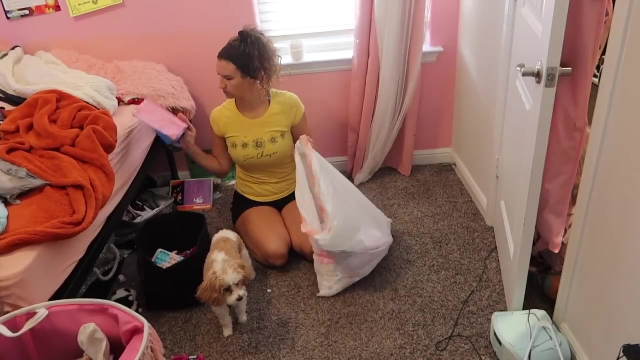 But I thought it would be helpful to share some tips and tricks of like what I do whenever I'm tackling a really big area like this one. You guys know, typically the other spaces in my house aren't this messy. This is very overwhelming. You feel like you have so much to do and you 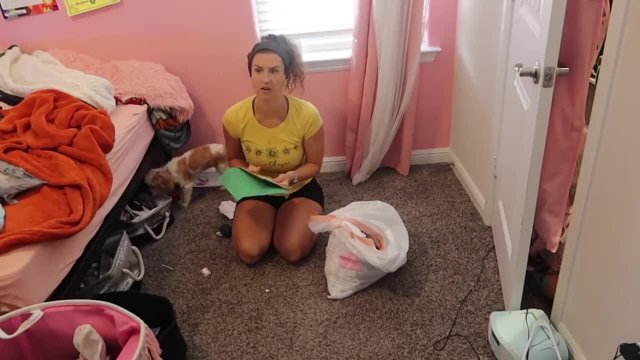 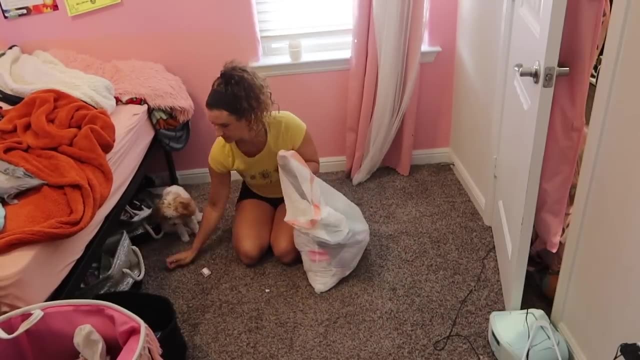 don't know where to start. So if you guys have somewhere that feels like that to you, don't feel discouraged or you keep putting it off just because it's overwhelming, Because I know it is tough, Like when you're looking at a huge project, it can feel daunting. 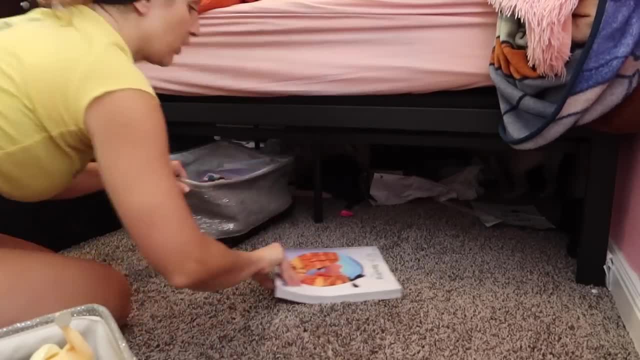 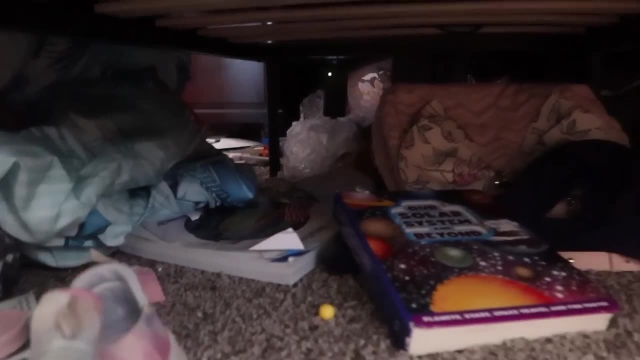 but I promise you can do it. You can get through it. Just focus on one thing at a time. So for me, like I said, I focus on trash. So number one thing is trash, If there's garbage in a space. 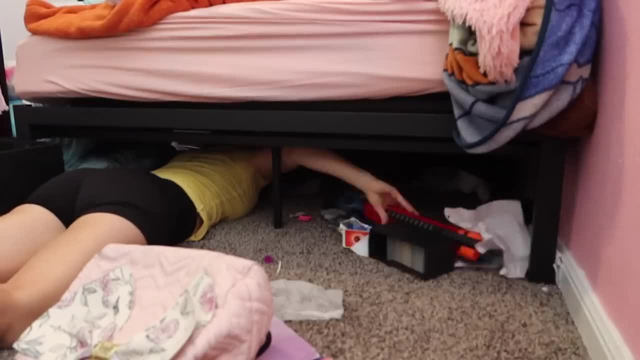 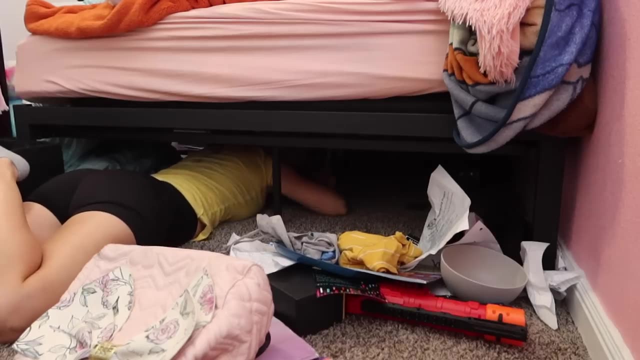 start with that, Just start grabbing all the trash out of all the spaces in that room and get that out of there first. Get rid of a lot of clutter and help your mental space a lot. So that's what I was doing. I was. 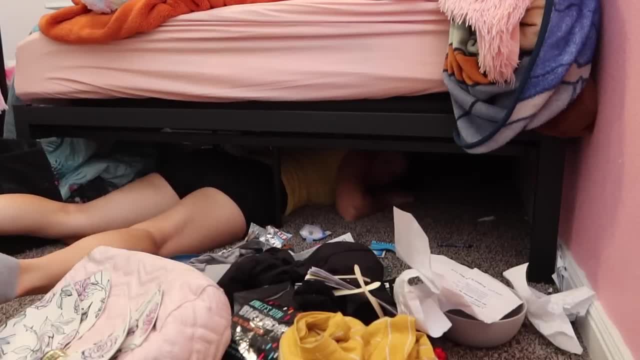 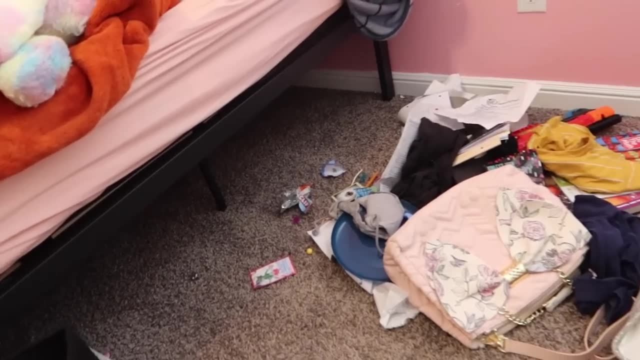 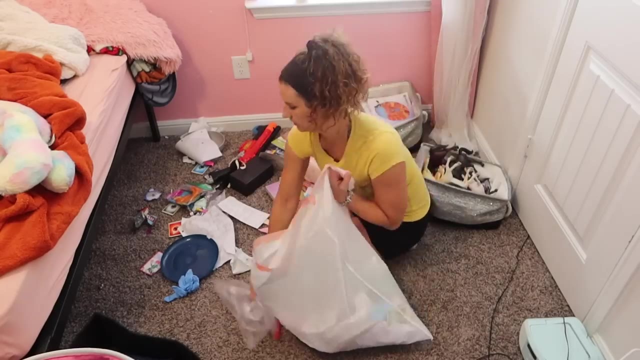 just trying to pull everything out from under the bed and throw away all the trash, And then we were going to get to the actual looking through things. And if trash isn't your problem, then pick one thing to start with. If it's a closet in the room, a drawer, a cabinet, start with one and completely. 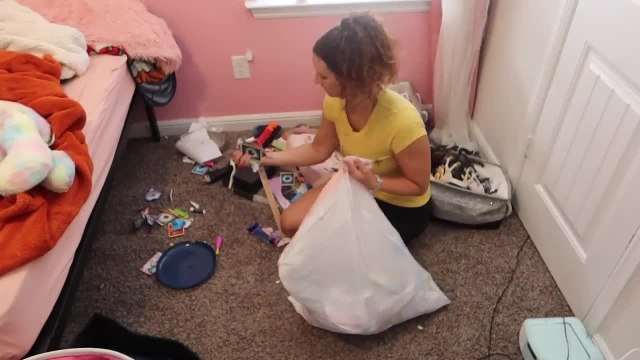 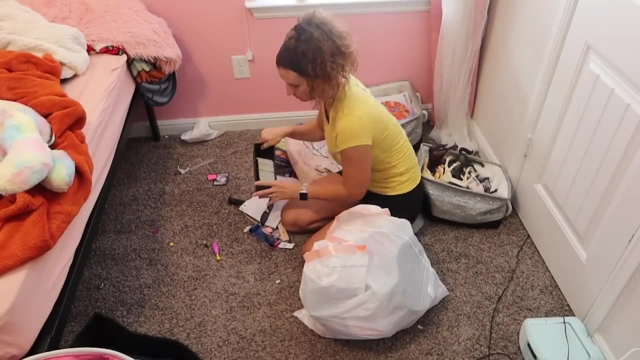 go through that And I promise that will give you the motivation to start with that To tackle the next drawer or the next cabinet. start small and build that motivation and stamina to keep going, Because once you see the progress you made in that one drawer or cabinet, it really 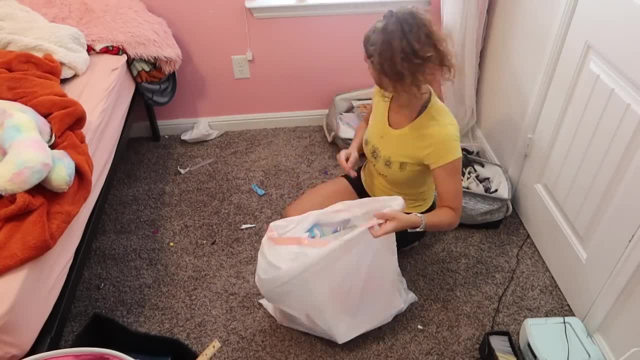 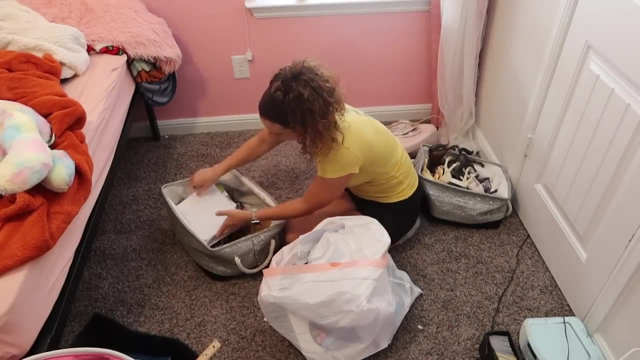 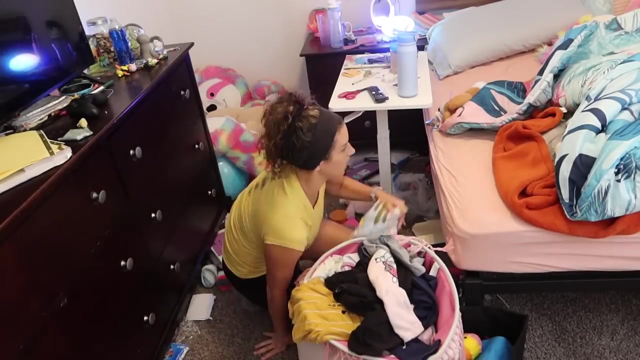 is going to give you that boost to keep going. I see you from across the room. It's kind of crowded here, but I know you see me too. Everybody's singing, Oh, everybody's singing, Oh. so I thought I would just put a little disclaimer in this video, because I always get comments relating to this. 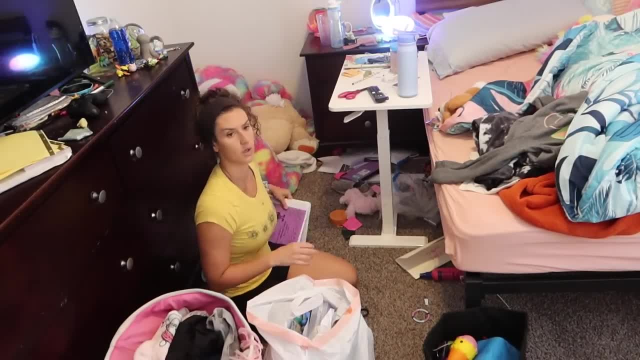 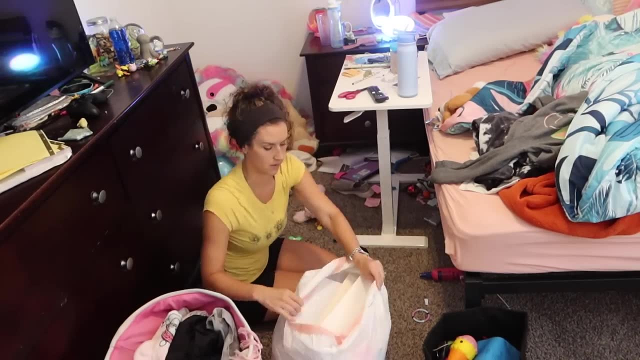 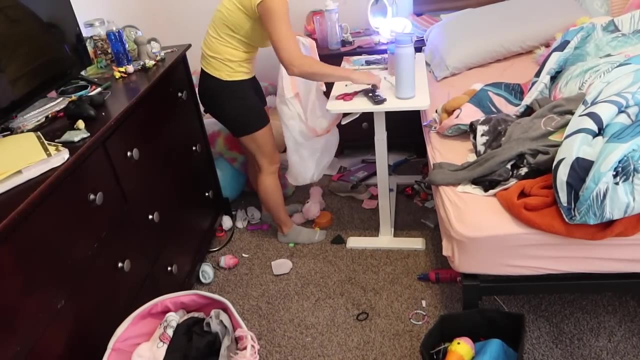 whenever I post Adrian's bedroom cleaning- and yes, she cleans her bedroom- I have them clean their rooms weekly and I do a check on Fridays and basically it's just: are the floors cleared and they have to vacuum? Those are the two things that I make sure the kids do And, as you can see, for 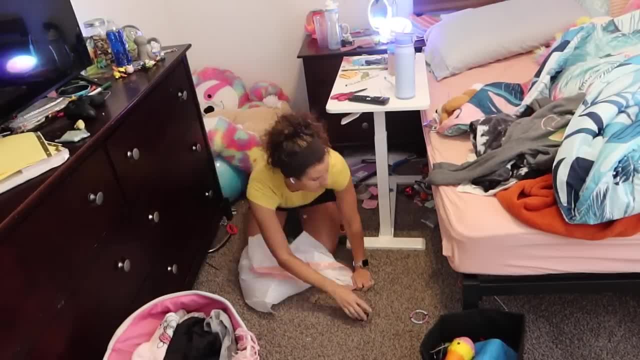 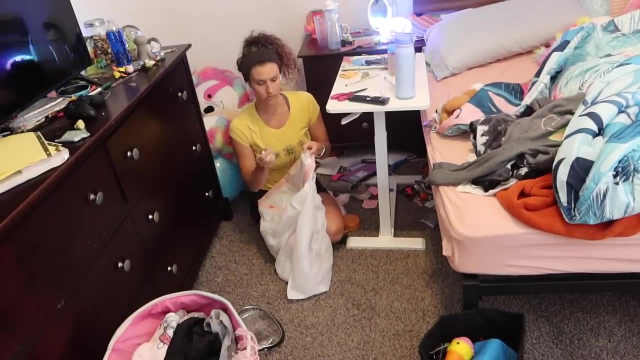 Adrian. she shoves things in drawers under her bed in her closet. that's how she cleans up. So every once in a while I'll tell her: you need to clear away your dressers, You need to get rid of the trash. But for the most part 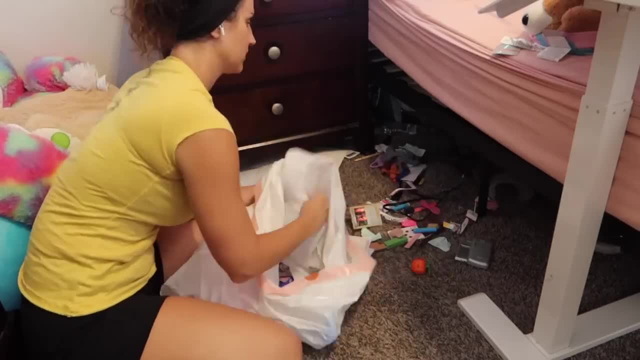 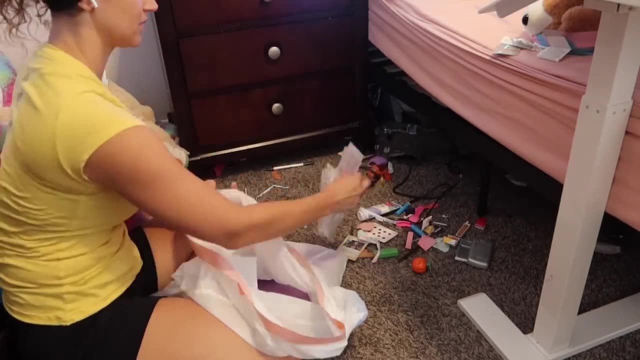 I'm just picky about cleaning up the floors and vacuuming because I want to keep the dust up. Obviously we have animals and everything, so she does clean, but it's definitely not my type of cleaning. My kids do have chores, but I do have to clean up the floors, So I'm just picky about. 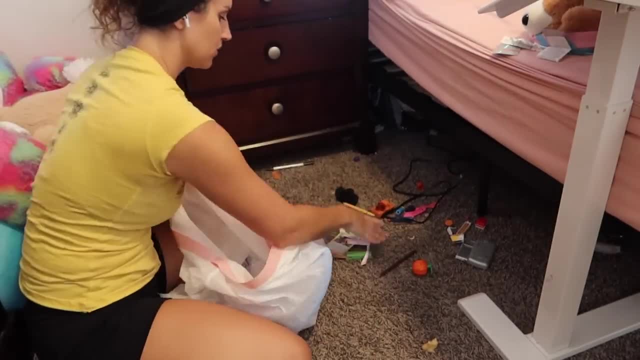 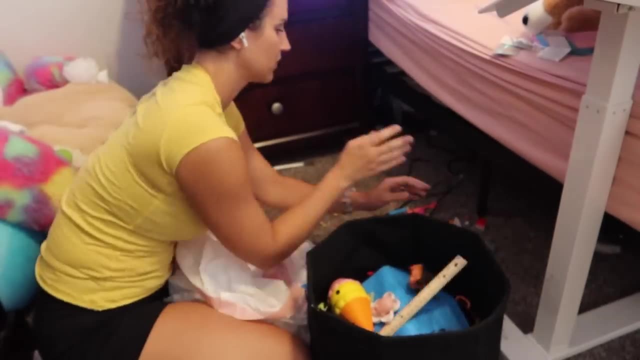 cleaning up the floors and vacuuming because I want to keep the dust up. Obviously we have animals and I do a deeper cleaning in her bedroom. I'd say once every month to two months So you can see how messy her room got. I want to say it was almost two months since I've done the last one. 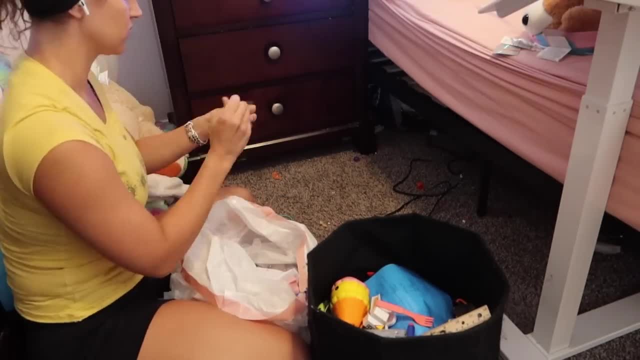 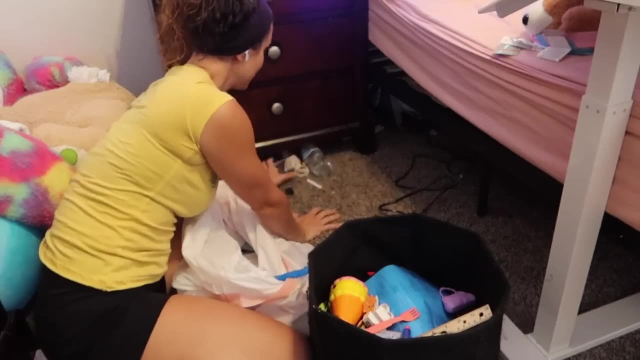 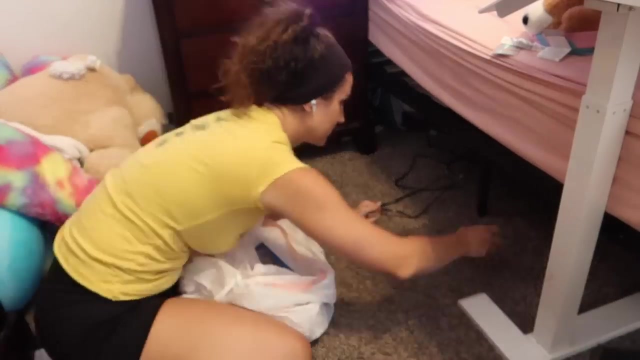 I'd have to go back and look at the videos, but she definitely can accumulate a mess quickly, which I feel like. every child is so different And I feel like before you hop on here and be a keyboard warrior, you need to remember that every child is unique and they 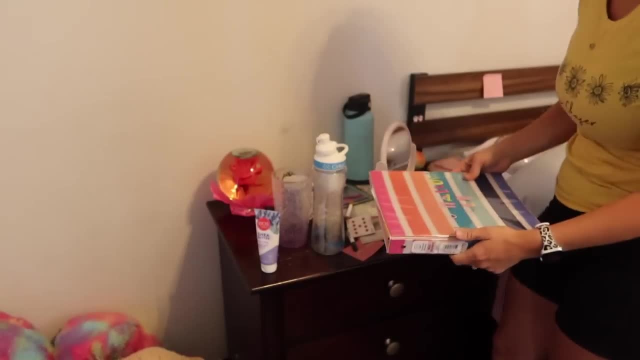 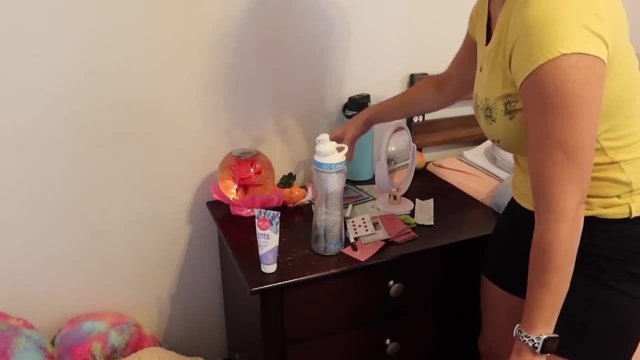 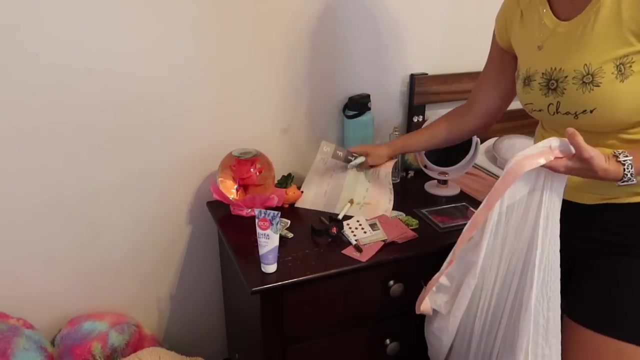 they thrive in different atmospheres And my job as a parent is to make sure they are healthy and happy and live in a safe space, And those things are definitely a priority to me, And having a immaculate bedroom is not a top priority for me. If she doesn't mind clutter, then she can do her. 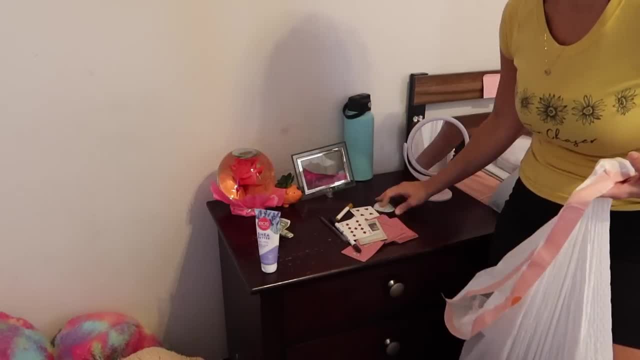 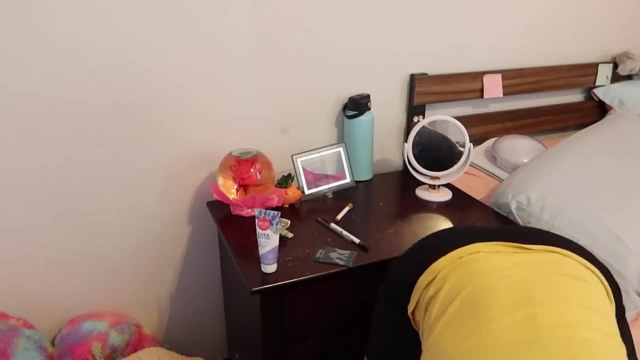 this is her room And you know I just make her keep up with her mess and then go in and help her Every once in a while, And that is fine for us and our family. And if you don't like that, 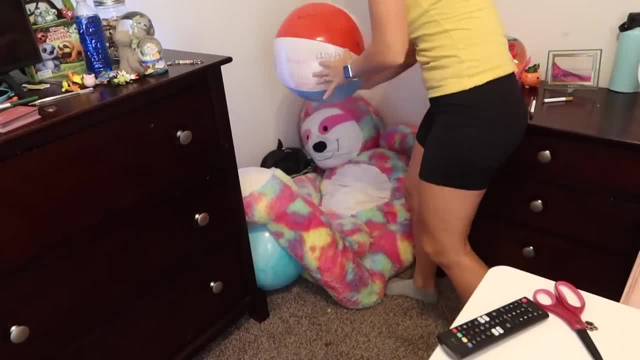 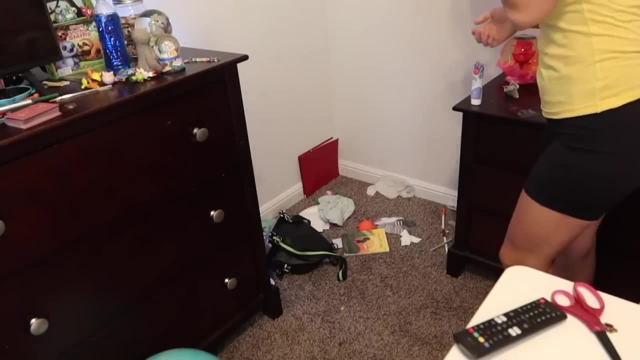 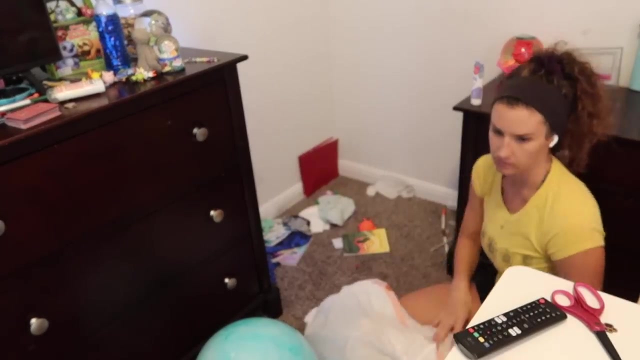 or you have different standards in your home. that is completely fine, because that is your home And this is ours. So I just ask that you guys be respectful whenever leaving comments. I don't know what it is about you. It must be in the way you move. Just say you want me to. 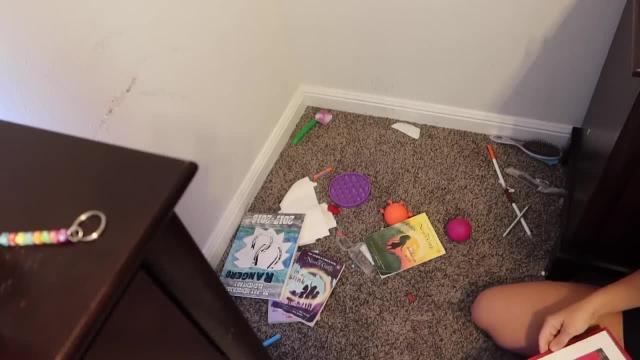 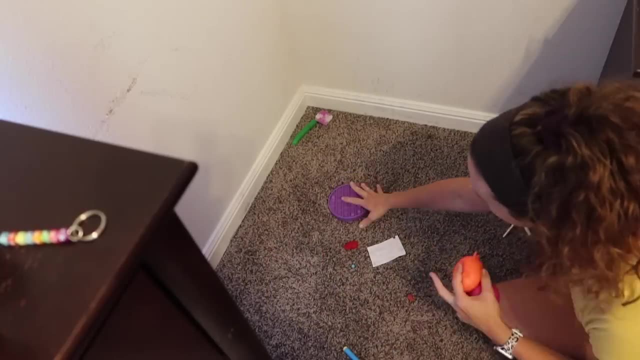 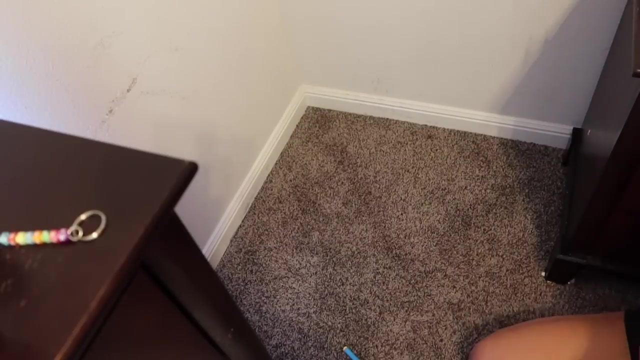 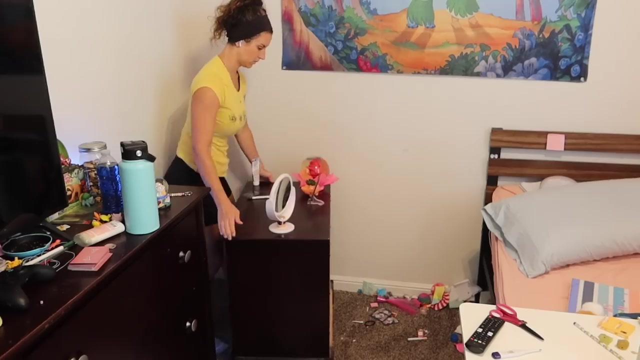 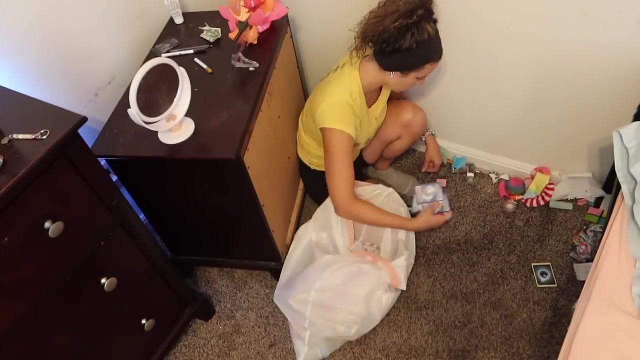 we got. I was finally starting to feel like I was making some progress. At first, I just felt like I was moving the clutter from one spot to the next, but I'm finally getting somewhere. We're going to go ahead and move the. 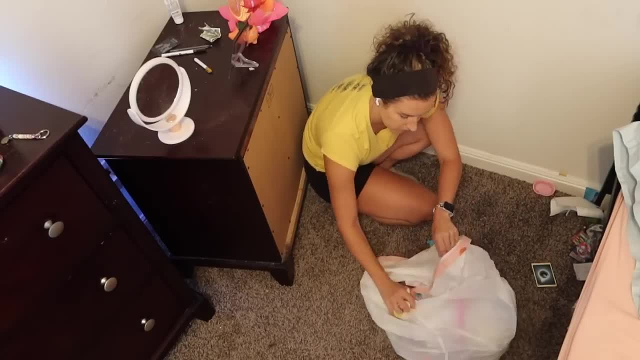 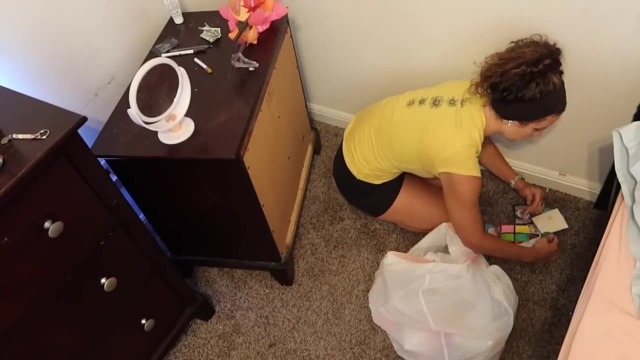 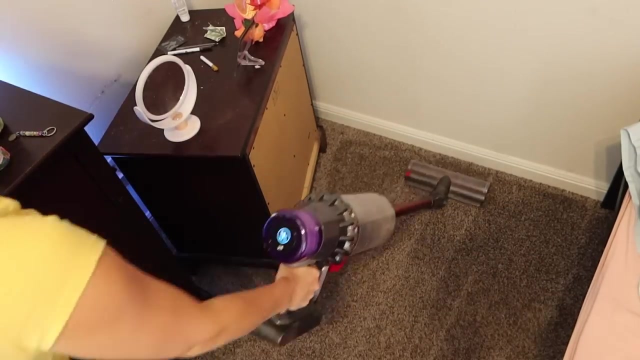 nightstand, cleaned underneath of it And then we're going to go through the inside. The drawers basically just had all of her Pokemon. My kids are huge Pokemon fans, So she has a lot of tens of Pokemon and I wanted to make sure I just gathered it up and put it into the closet instead of the. 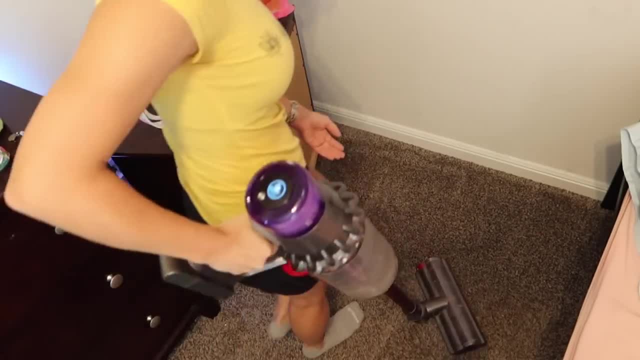 nightstand So we could get this out of here. I haven't quite decided yet if I'm going to hold on to the nightstand and maybe redo it or not. I will be able to do that in a few days. I'm going. to be able to do that. So we're going to be able to do that in a few days. I'm going to be able to do that in a few days. I'm going to be able to do that in a few days. I'm going to be able to do that in a few days. 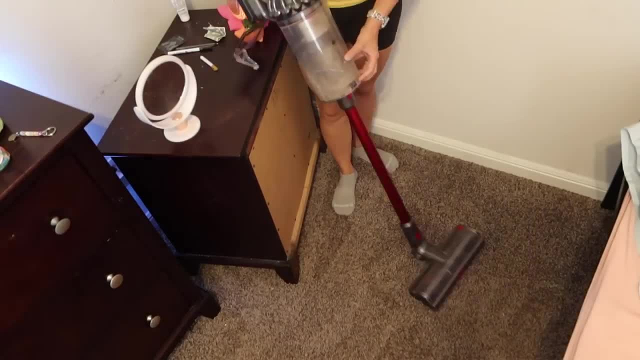 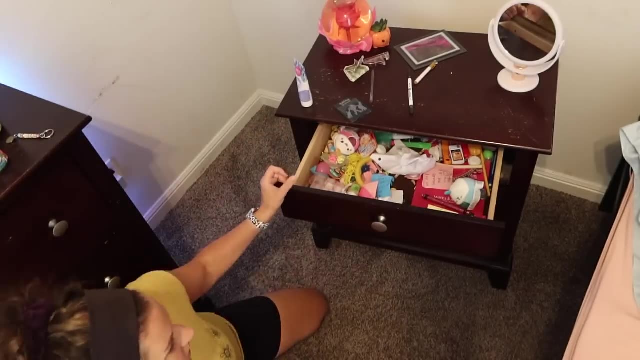 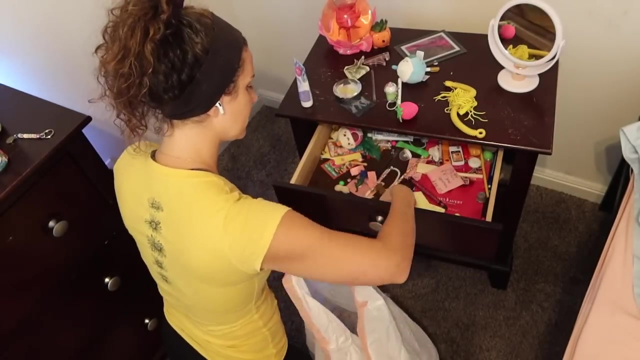 stand and maybe redo it, Or if we're just going to sell it, because I mean, as much as I love DIY projects, honestly I just never really do them. Like I have to be in the mood and I feel like we already have so many things in our storage that I'm just kind of leaning towards selling it. 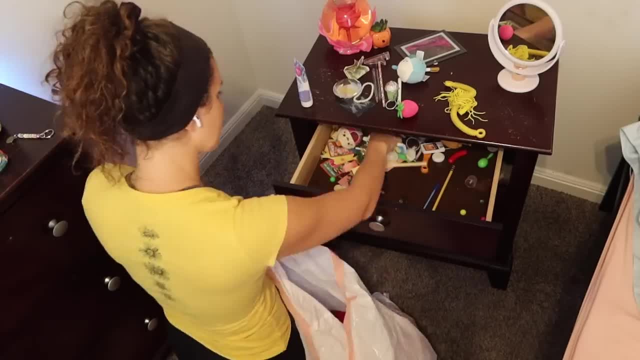 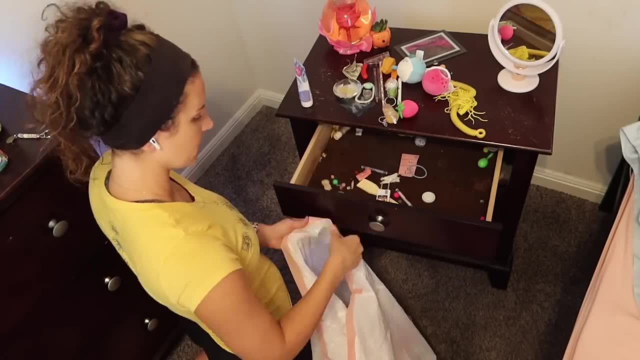 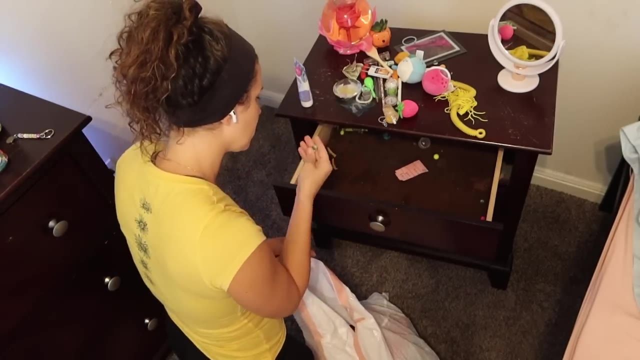 But random fun fact: the furniture in her bedroom- So the nightstand and the dresser with the mirror on it- is actually the first furniture that me and my husband purchased together, So it definitely holds a lot of sentimental value to us. It is about 15 years old and it's definitely held up. 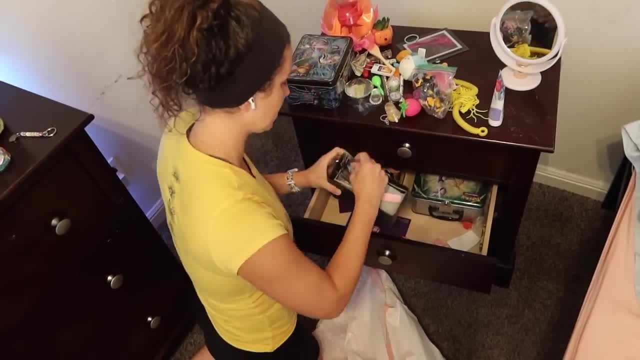 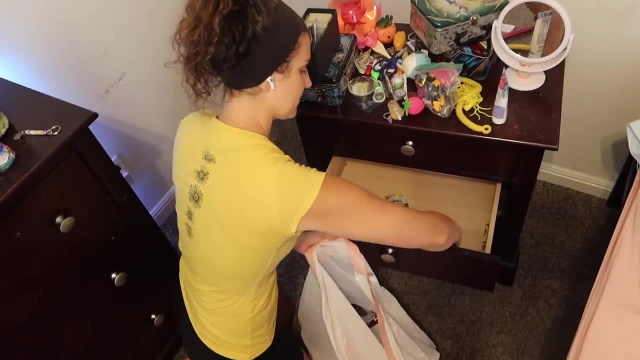 We got our money's worth. but that definitely makes me a little sad when I think about selling it, because I'm like man, we've had it for so long and I don't know. So we'll see. We'll see if I sell it or if I'm going to redo it. 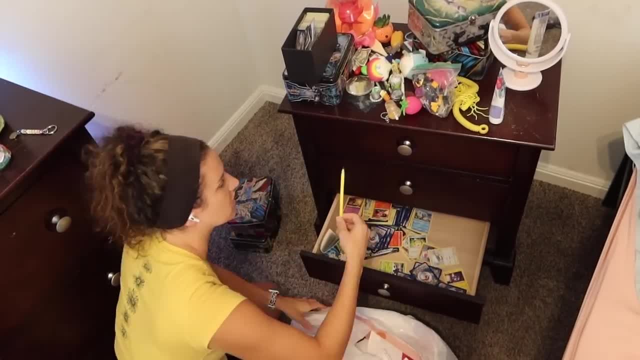 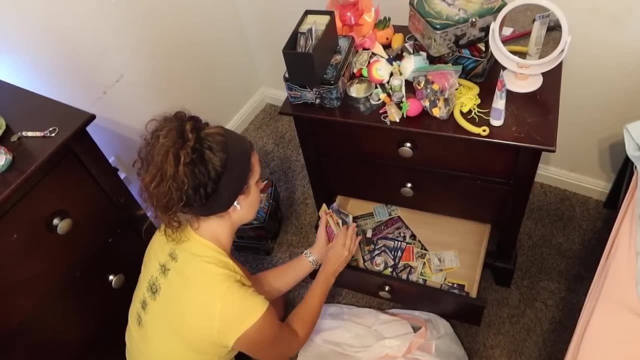 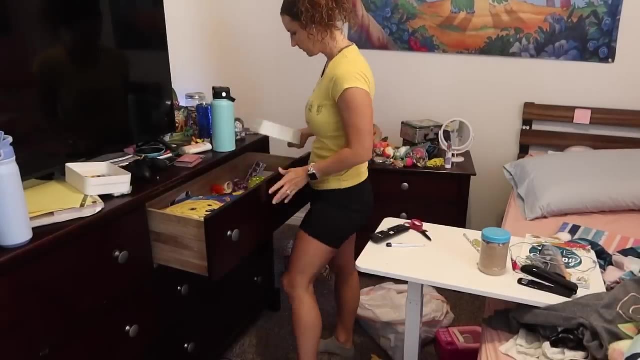 But I can't believe we've had this furniture for 15 years. It's just crazy how fast time goes. Me and my husband are actually about to have our 15 year wedding anniversary, So that is, on August 11th It'll be 15 years of marriage, which just blows my mind, You guys, I don't know like. 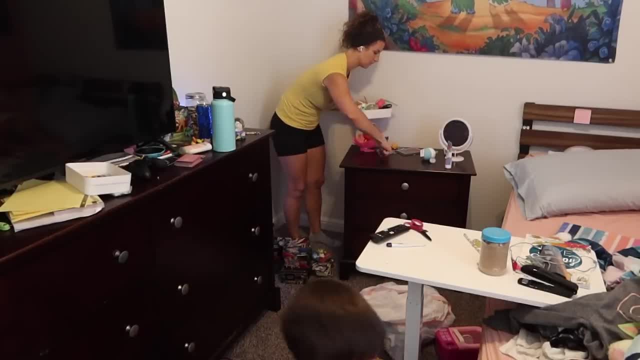 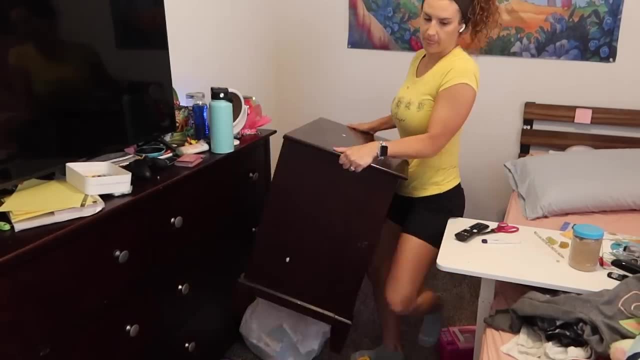 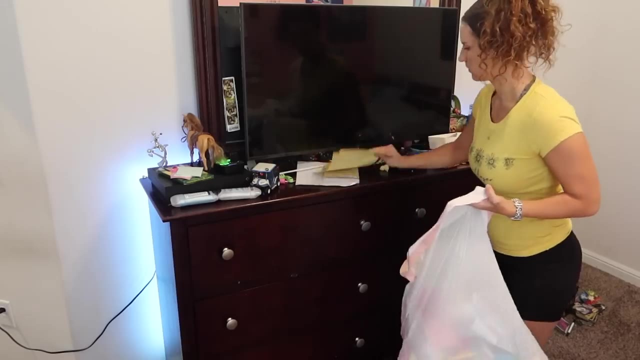 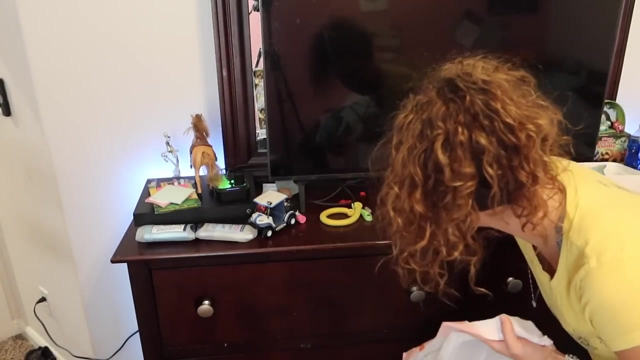 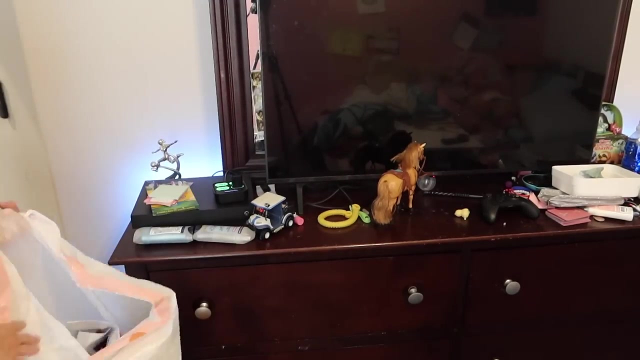 where the time goes. It's crazy how, once you have kids, it's just it just starts flying by. I'm quickly going to go through the top of her dresser and just get rid of all of the trash. I'm going to be leaving the toys and fidgets because she will be going through those. 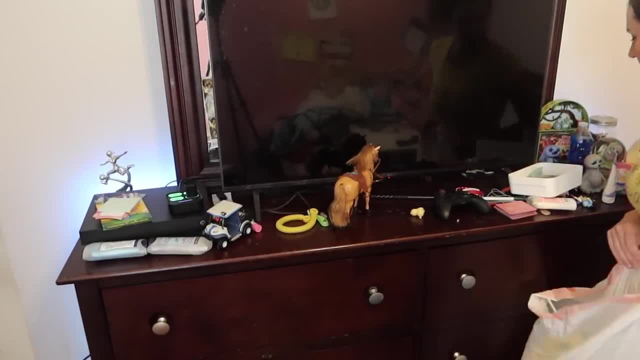 and discarding whatever one of them she wants. So I'm going to go ahead and get rid of all of the toys and fidgets, because she will be going through those and discarding whatever one she no longer wants. But I just needed to get the trash off of here before I moved the dresser. We 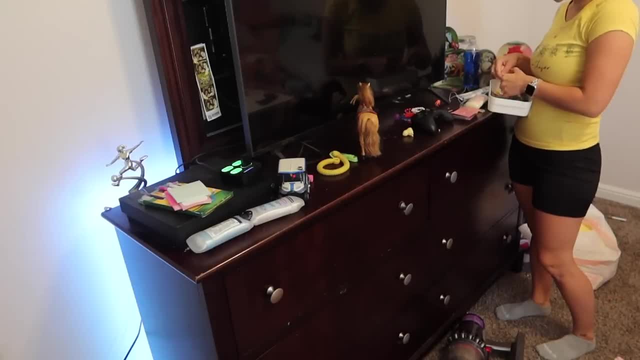 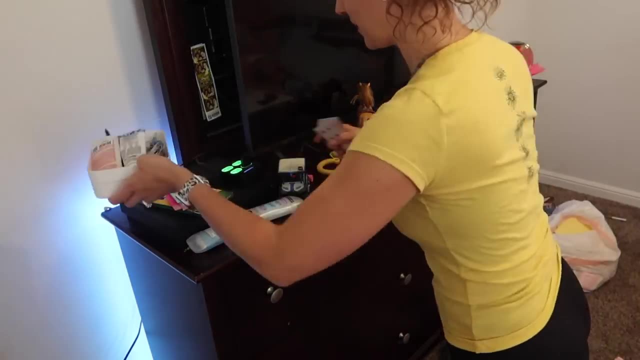 definitely needed to clean underneath of it because there was so much trash under here. And then I'm actually going to be taking the mirror off of the dresser, because the mirror is pointless. I mean, you can't even see it because the TV is covering it up and Adrian. 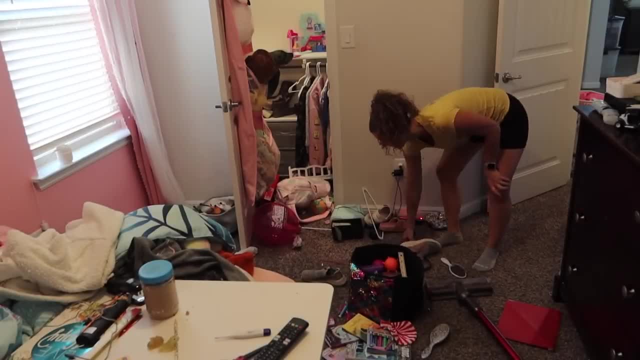 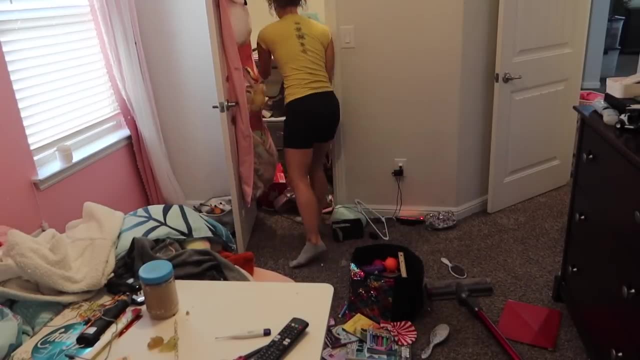 is always playing Xbox with Austin. So I was like you know what? I'm just going to go ahead and take the mirror off. It makes the room look less cluttered Without the mirror, like I knew it would make a big difference. So we're going to go ahead and 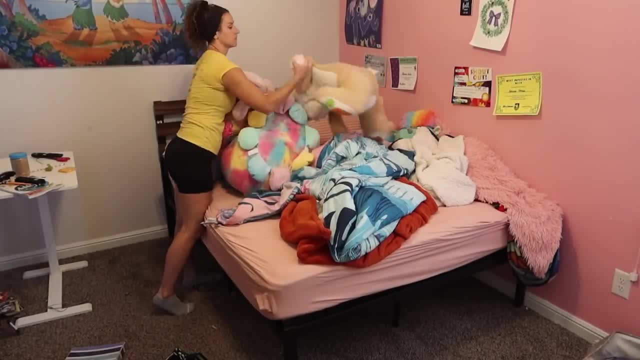 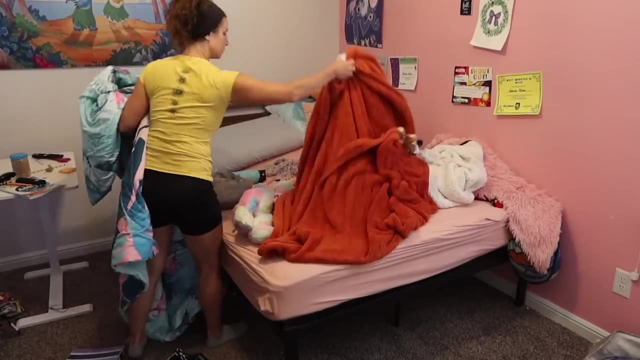 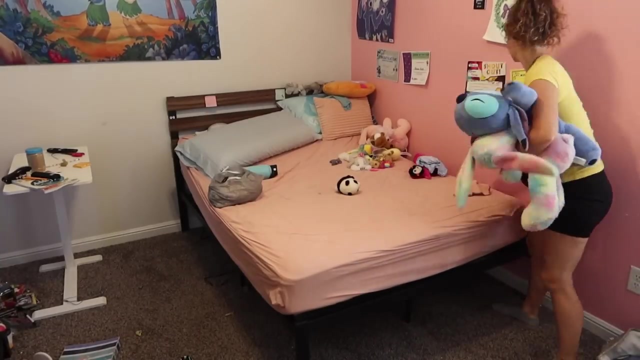 take that mirror off. whenever I move the dresser away from the wall, I'm alive and I'm breathing, living my best life. Love is on my mind and it's making me high. I'm staying in this moment, though it's hard sometimes, but I work it out every once in a. 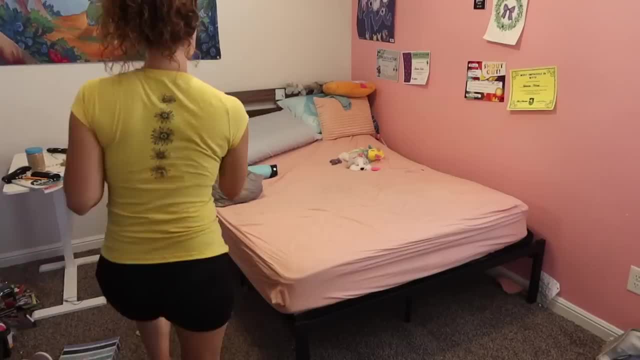 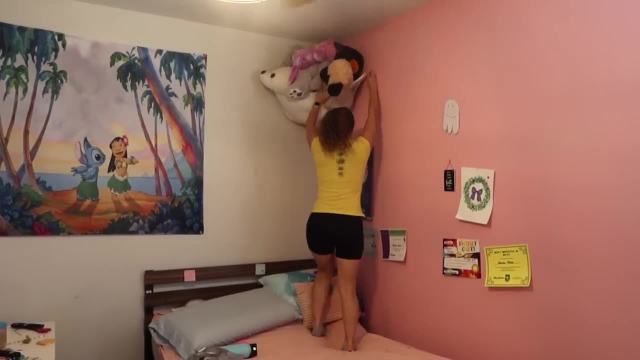 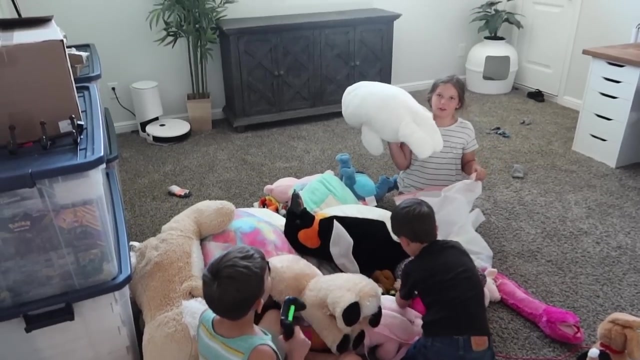 while I feel the love. You guys know that Adrian loves her stuffed animals. We have a corner, we have an organizer on her closet door and her bed is completely covered in them. But, like I told her, you know we have way too much in this room. She's been complaining how 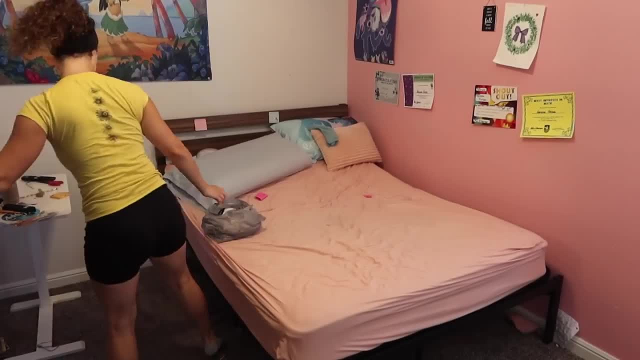 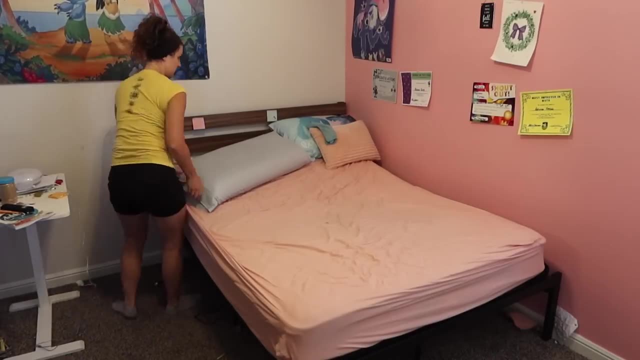 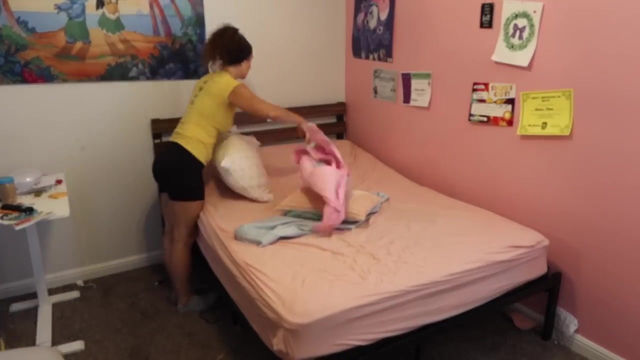 hot she gets. So I told her: you know, it's really time to get rid of some. you have a lot and make room for some more. So she was finally open to getting rid of some of her stuffed animals and finally getting rid of that huge sloth. You guys, that thing took up so much space in her. 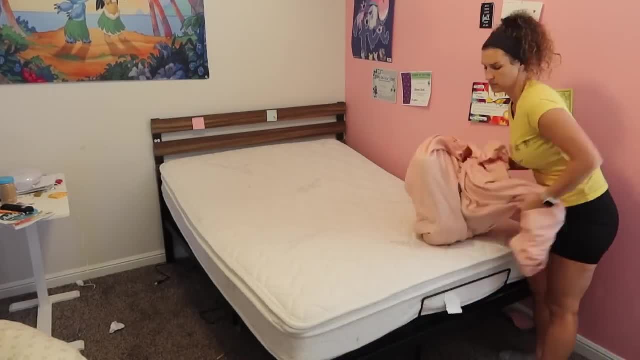 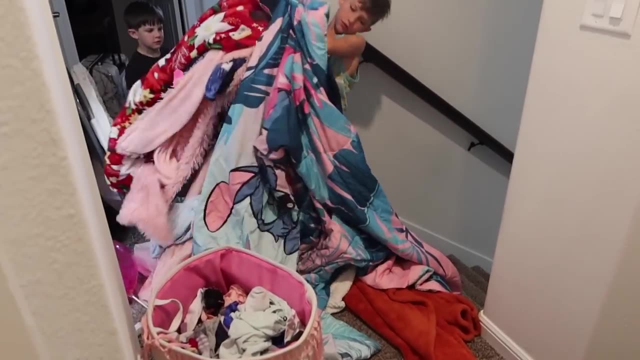 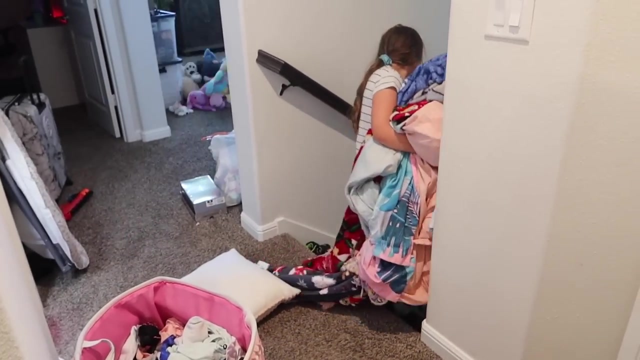 room. I was so happy that she finally was ready to let go and get rid of it. And once I pulled everything off of her bed, I realized that she had a big ink stain on her sheets. So I did try to wash them and get it out, but I could not get the ink to come out, So I will definitely have to. 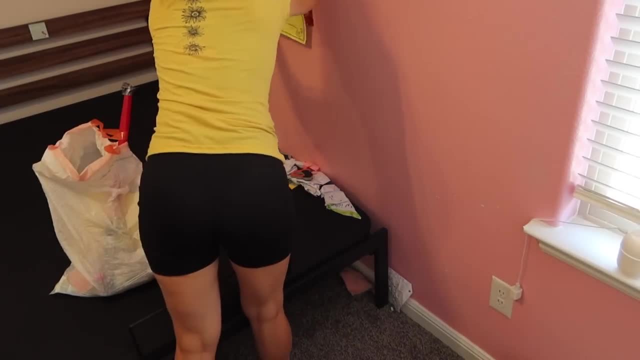 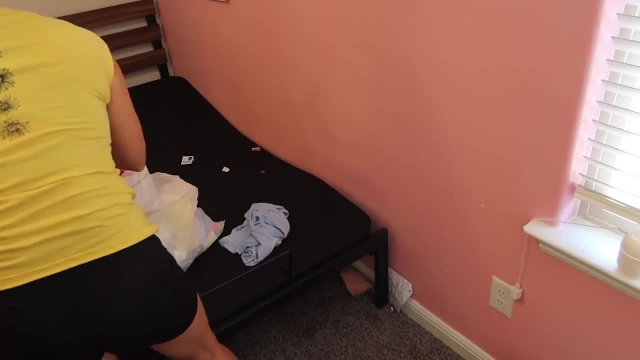 be looking for some more sheets for her to go on her bed. But, as you guys saw, we got her old mattress out of here. It was just like a cheapo mattress that we bought off of, So we were so excited to be putting the Lowell mattress in here. Adrienne was driving me nuts. 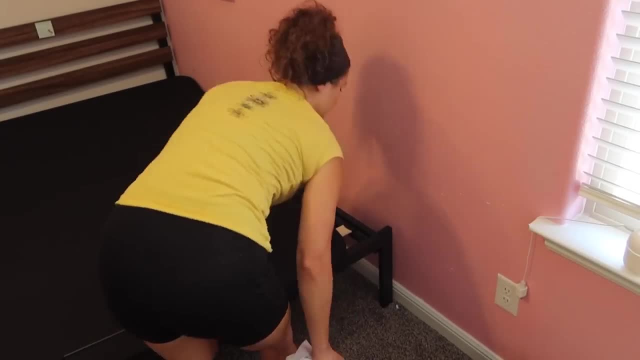 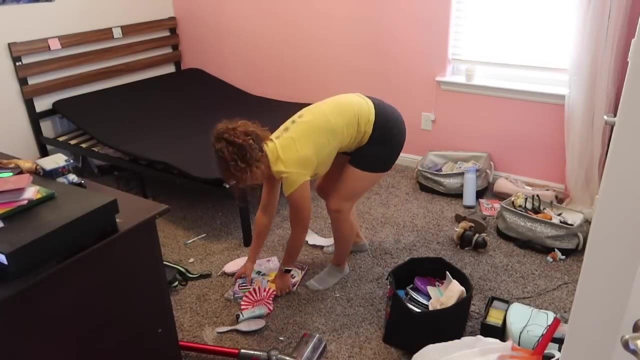 Like we have had that box sitting downstairs for a couple of days because I knew I needed to clean her room before we could set it up, And she was bugging me every day Like, mom, are you going to do it, Are you going to do it? So she was super excited about her new mattress. 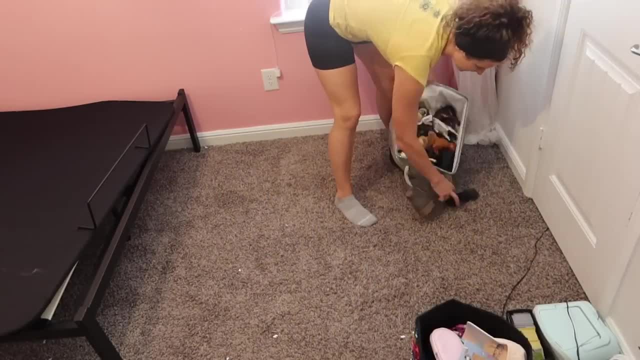 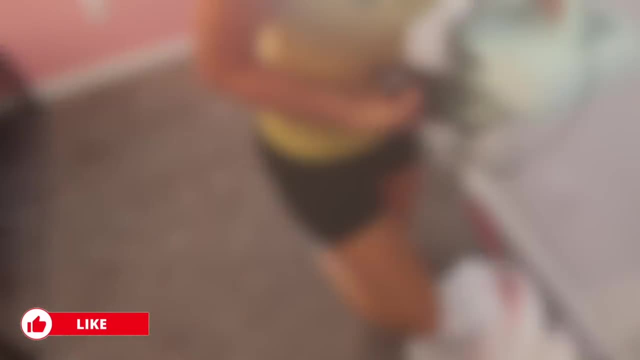 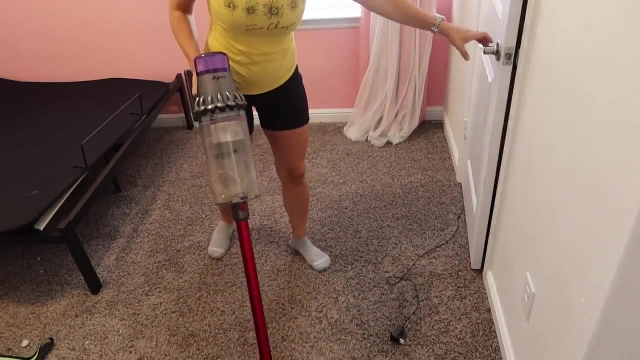 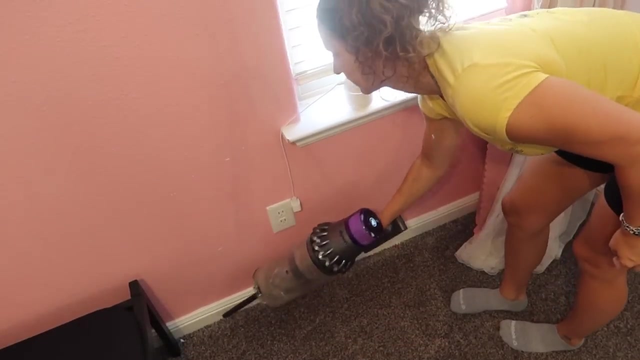 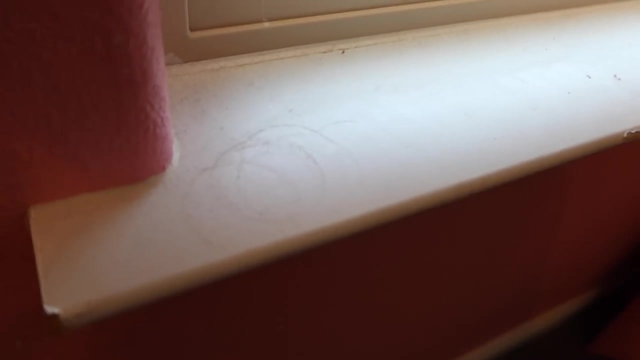 As I'm cleaning the room, I'm making sure to not only dust but wipe down the floor. So I'm going to wipe down the floor. So I'm going to wipe down the floor, The baseboards and the windowsills, just to make sure everything is dust free. 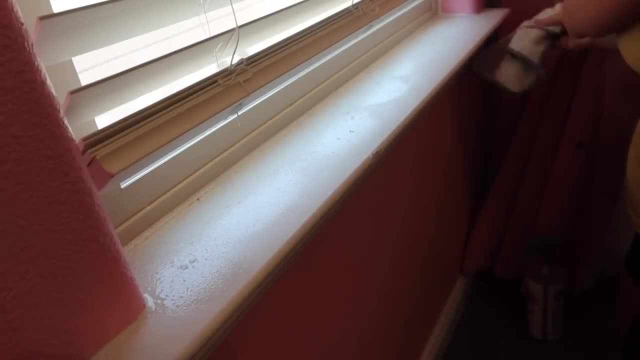 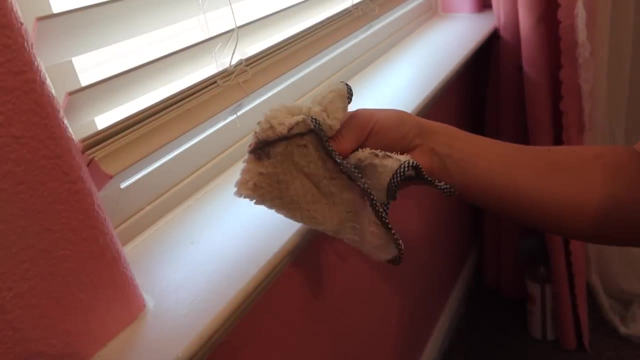 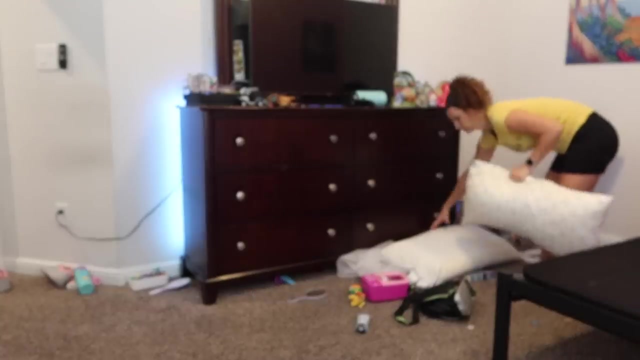 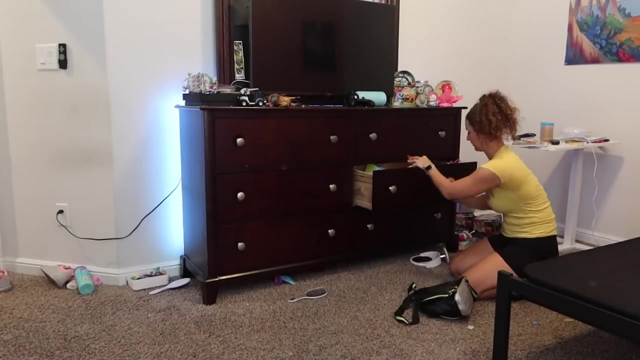 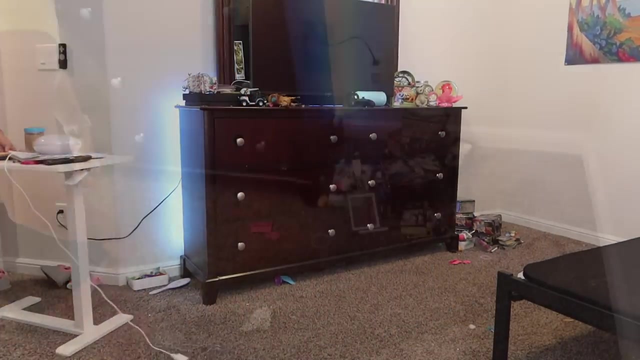 especially whenever I rearrange furniture, I like to do a deeper cleaning in the space, because you never know when you're going to see that baseboard again if you end up putting furniture in front of it. This is everything that we're going to be keeping. that came out of her nightstand. 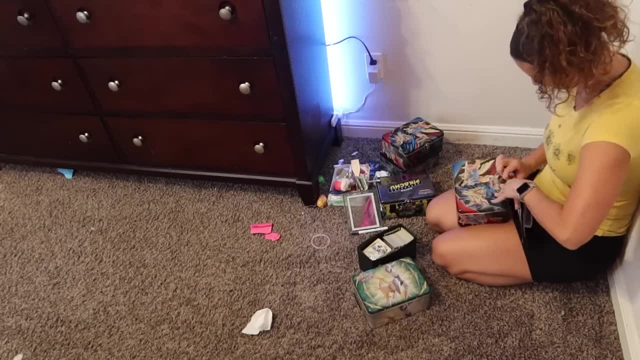 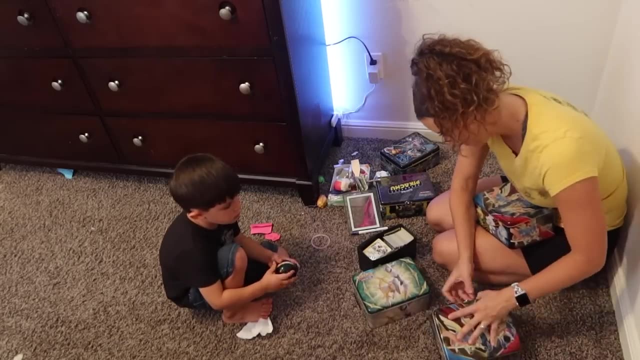 which is basically just her Pokemon. So I'm going to organize it really quick and then go ahead and just set it inside the closet, because I have not even attempted to start cleaning the closet. We're going to save that for after the bedroom is finished. 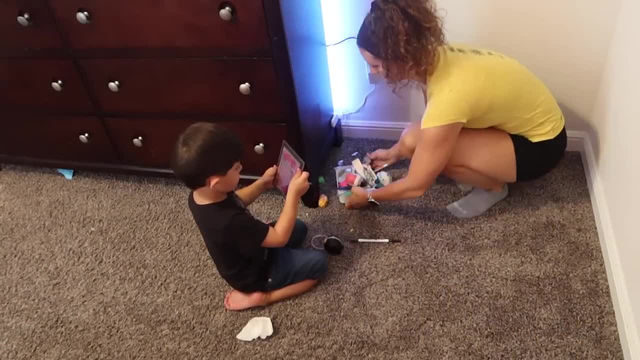 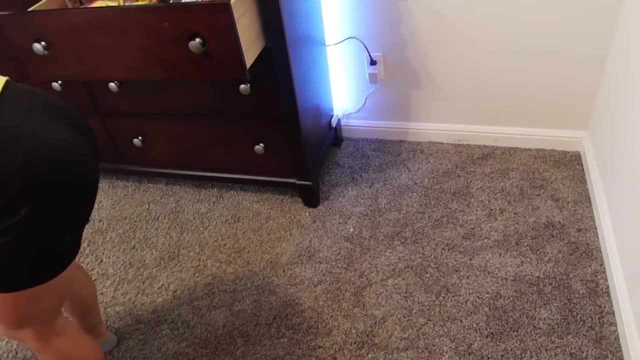 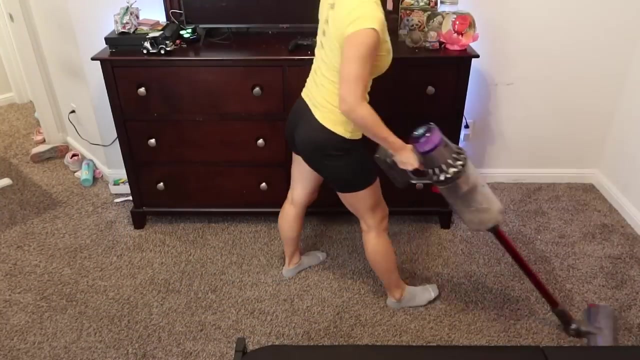 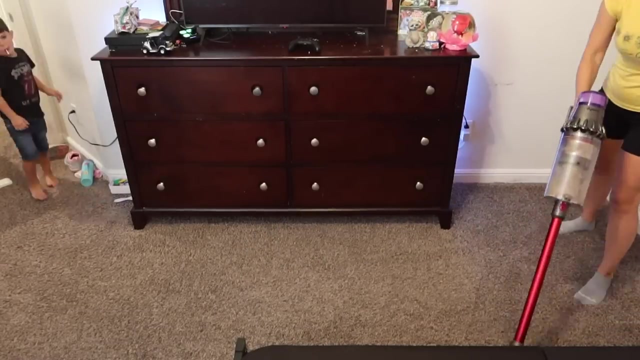 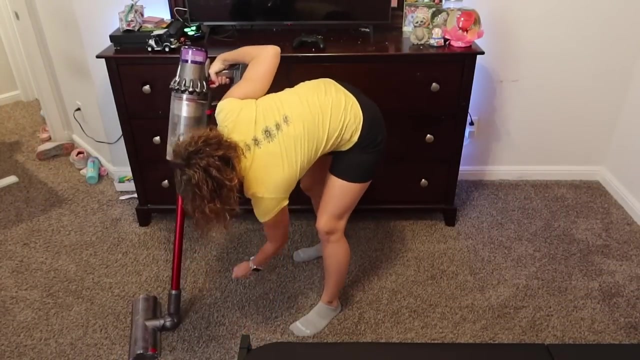 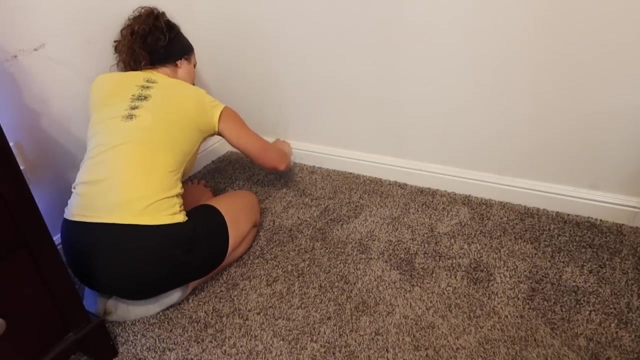 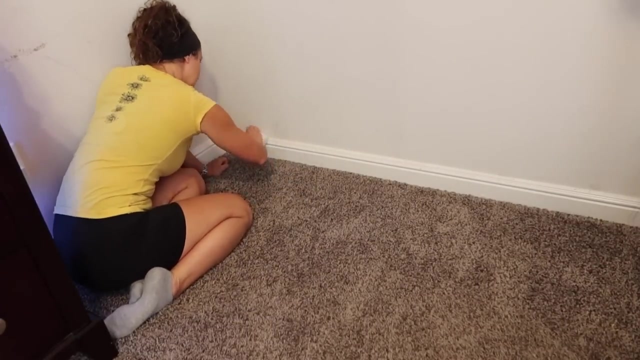 So I'm just going to set it in there and then find a home for it once we get into the closet. This poor corner is so scuffed up, So we used to have her little chair in this corner and I guess she had leaned back in it one time and it smacked the wall And, as you can see, there's like drywall. 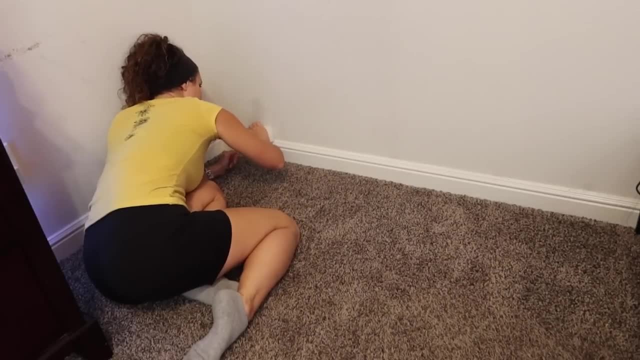 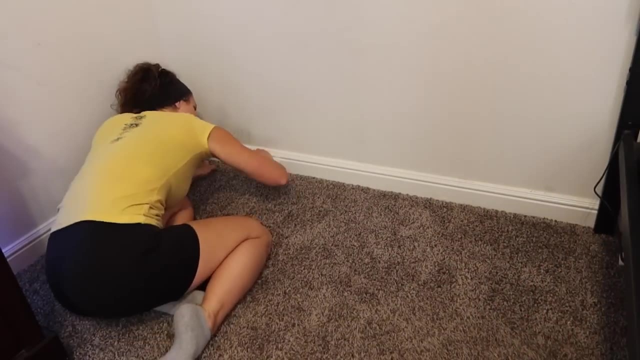 coming off. where it hit the wall There was these black marks on the wall. The baseboards need to be touched up. I did go in with my magic eraser hoping to get it off a little bit, but it just started to take off the paint, So I started to clean it up a little bit. So I'm going to 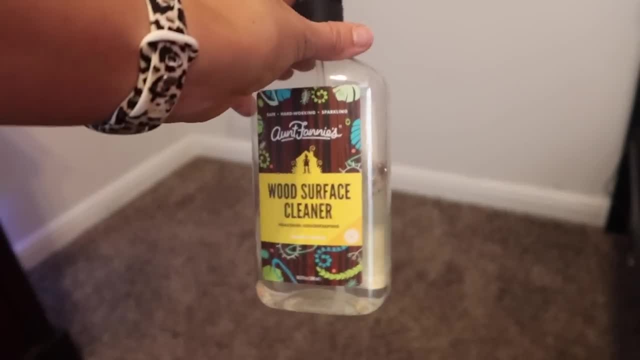 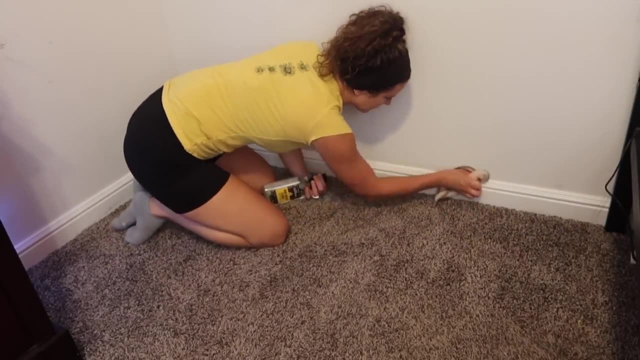 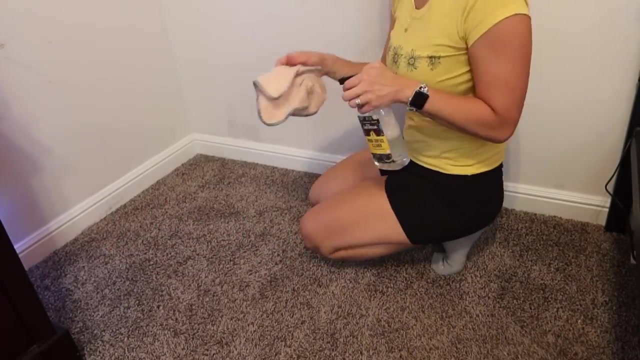 stop. I was like Nope, not doing this. I am going to clean the walls with my wall cleaner and then just clean the baseboards as best as I can, And hopefully I'll come in here and repaint the baseboards where they need touch-ups. But as for the paint, I don't know what I'm going to do. 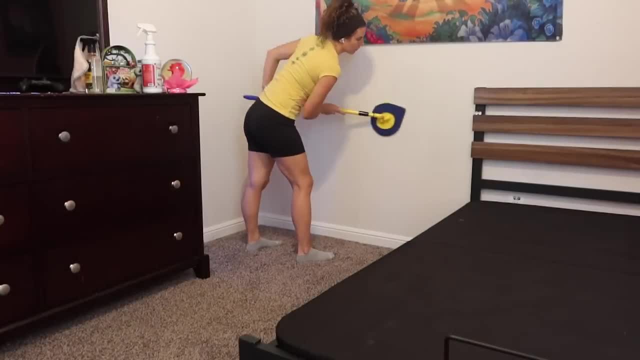 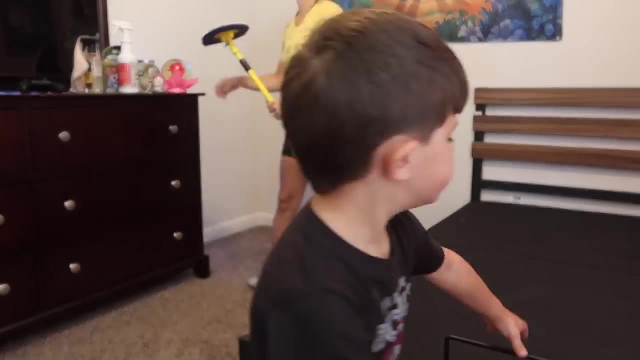 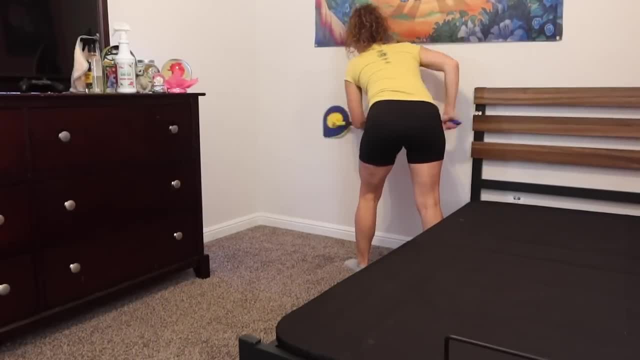 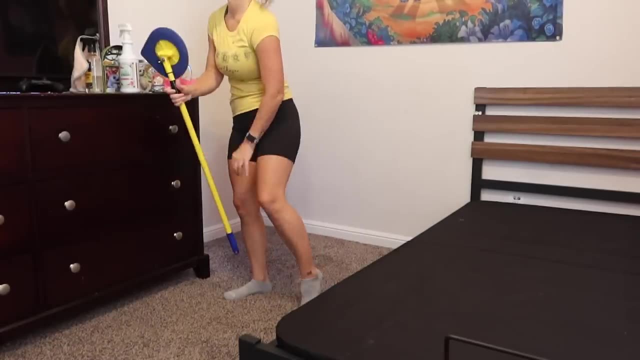 know what I'm going to do with it, But I tried to color match it like in the bathroom before I painted the bathroom and it did not match up. So I can't do like little touch-ups. If I want to like fix an area, I have to paint the entire wall. So maybe down the road I'll come in here. 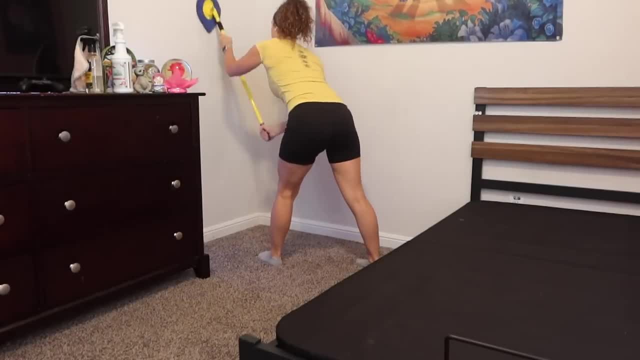 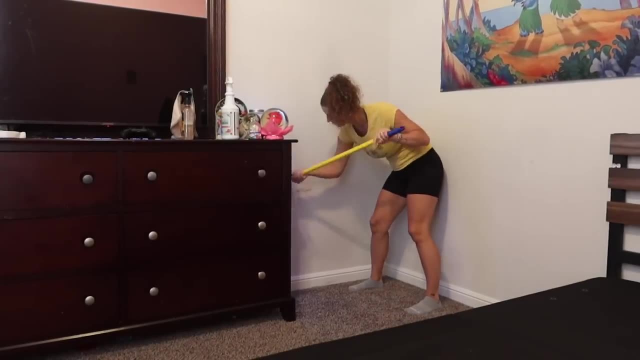 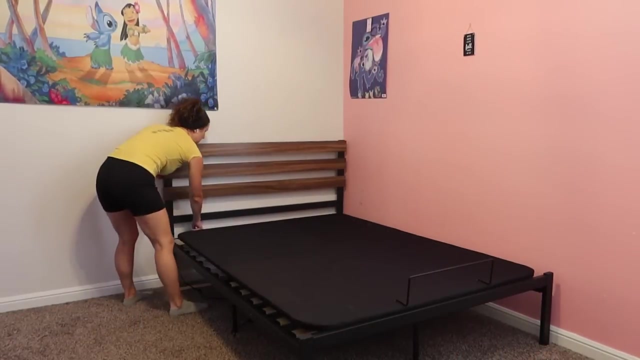 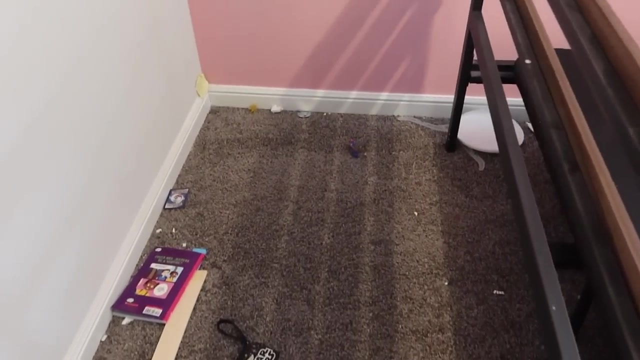 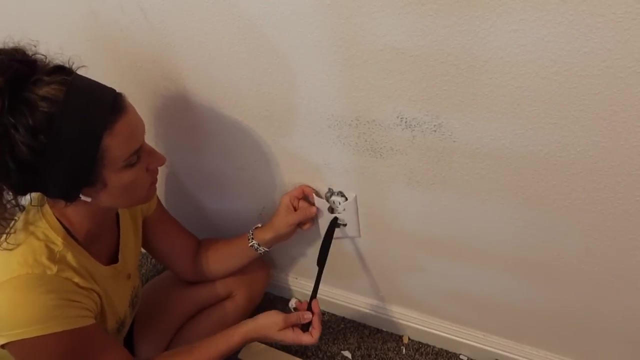 and repaint all the walls, because hers are really scuffed up. Once I pulled her bed away and started looking at all the mess underneath, I noticed that her outlet was completely crushed. So thankfully I had recently bought a bunch of um little outlet. 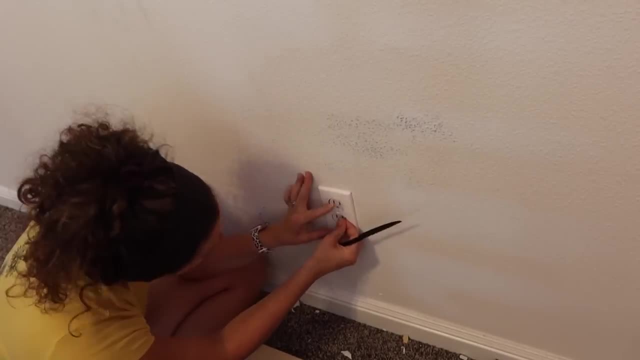 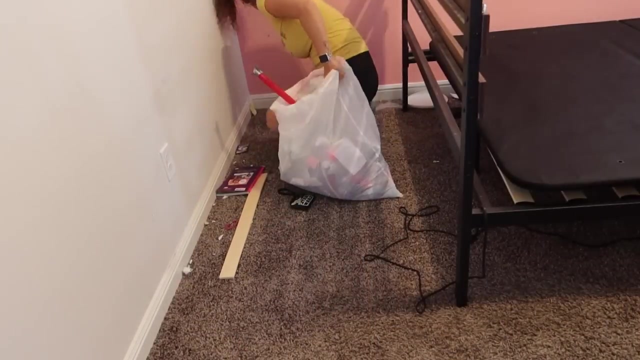 covers. I bought like a big pack of them, So I was able to go ahead and replace the outlet cover, And then we're going to clean underneath here And also wipe the walls as best as I can. The spray did a really good job at getting up a lot. 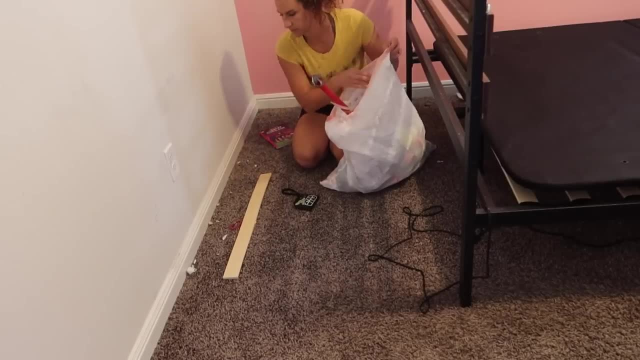 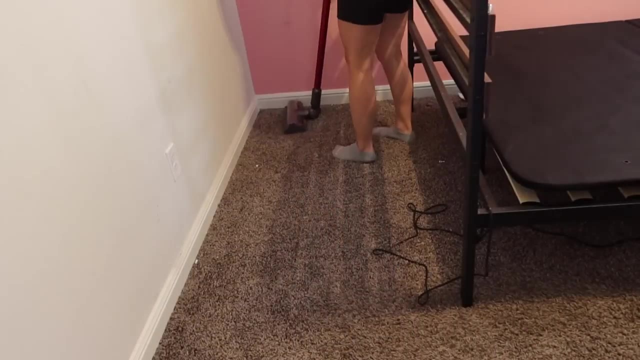 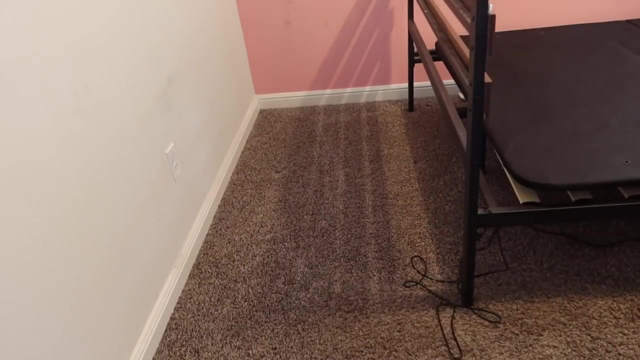 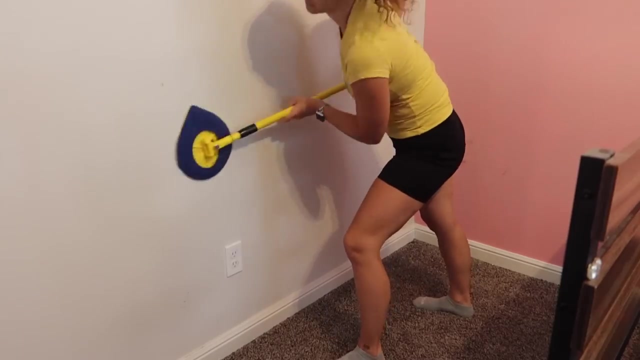 of the like, dirt marks and stuff. Obviously, the deeper scuff marks won't come off because I have flat paint, but it made a huge difference cleaning the walls. It looked so much cleaner in here. It's so awesome. Yeah, Yeah. 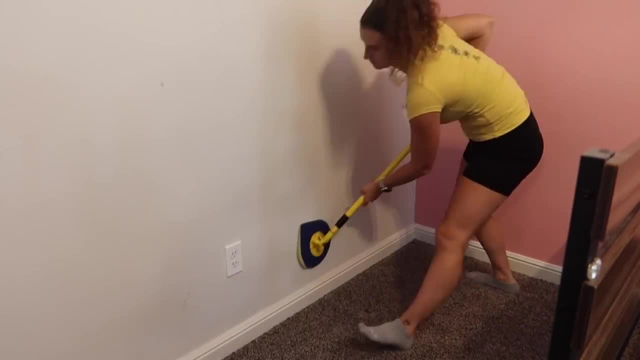 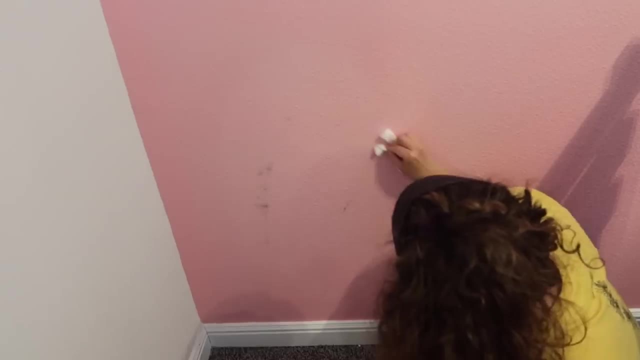 Trying to make it a little. mama, Doesn't matter how deep I go now You can lean on me like a ton of pizza. Y'all give me a piece of mind, like you were St Terese, But damn, you can also be a danger. 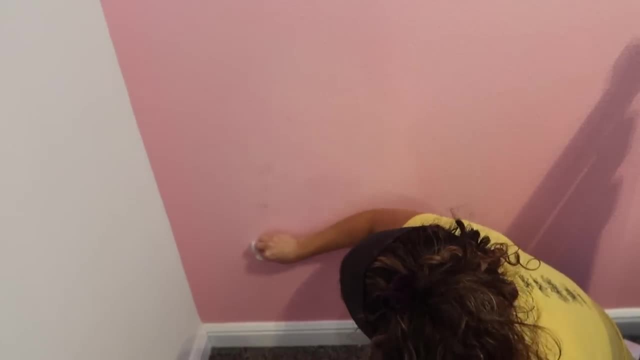 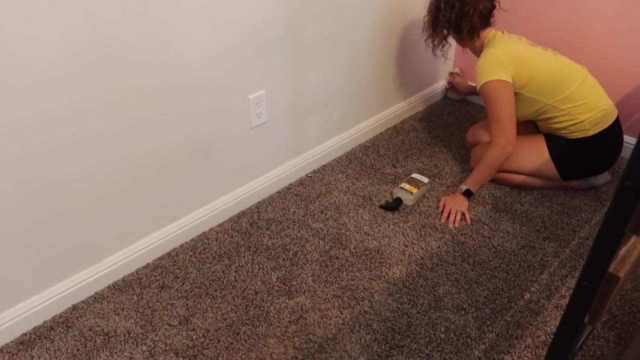 You're so dangerous, like wild savanna Playing with lava. Without that I can't take this anymore. I want to always be making love to you. You steal is a crime, Damn girl. you're fine When I'm with you. 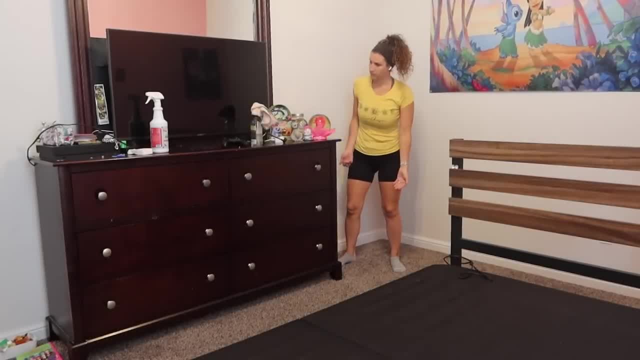 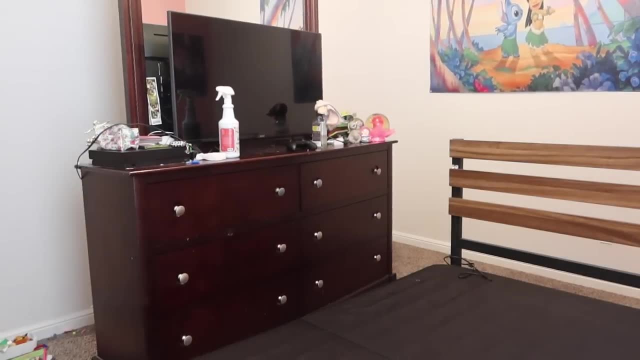 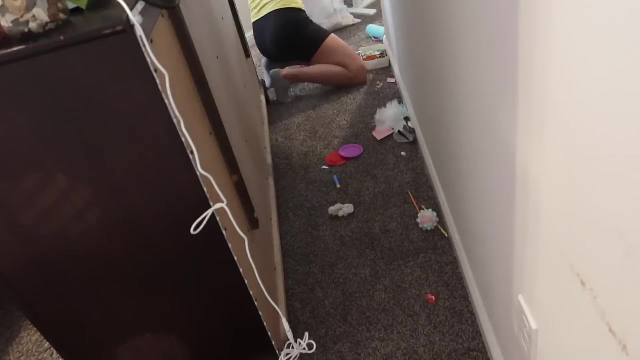 now that the floors are basically all cleared away, I can finally move this dresser out and start cleaning underneath of it and take down the mirror, and then we are going to be rearranging the furniture, which I was really excited to do. the way that I'm going to be putting it. we actually 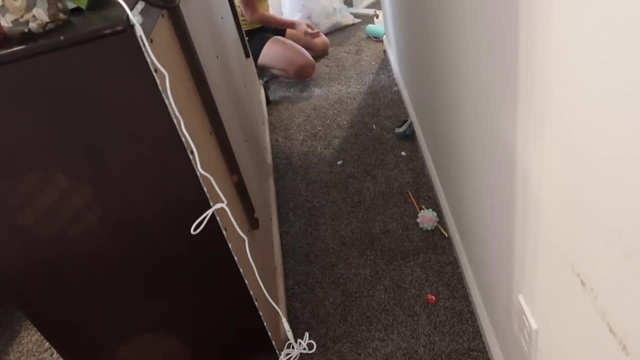 had her bed like that when we first moved in, but because of the nightstand and everything it just looked super cluttered. so I was excited to rearrange it without the nightstand and just see how open it was going to look. rearranging furniture is one of my favorite things to do. 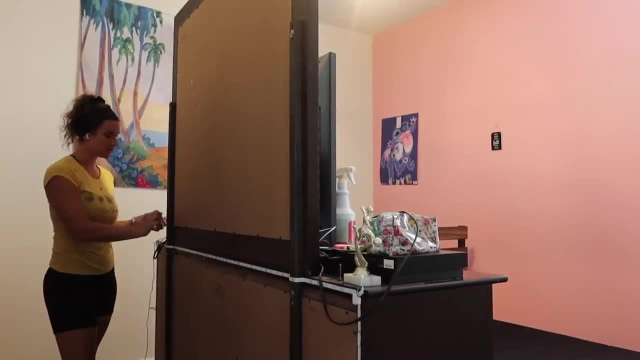 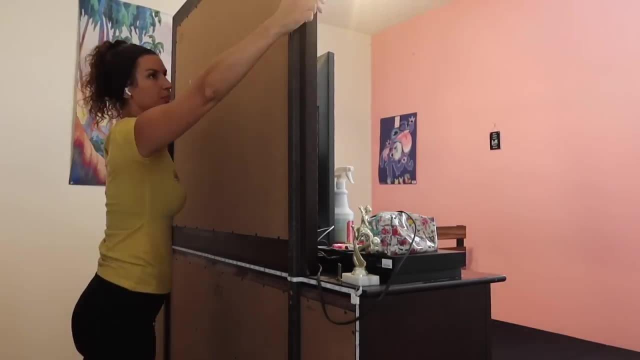 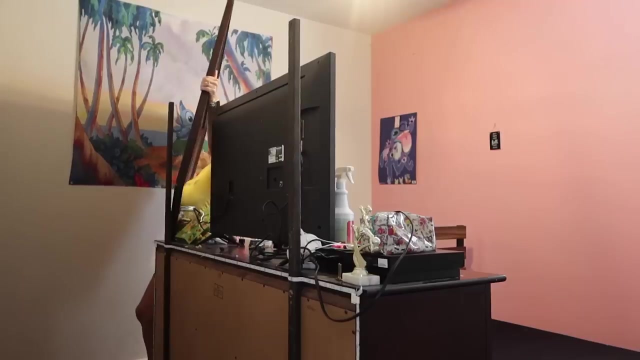 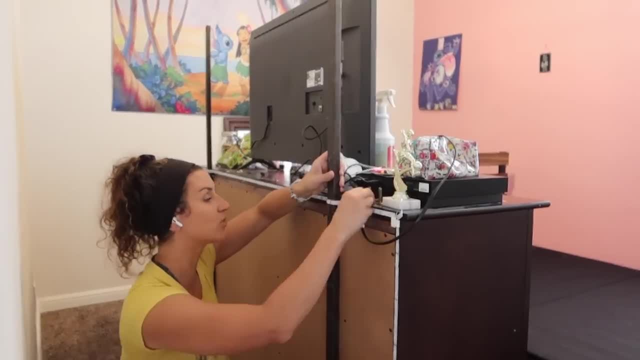 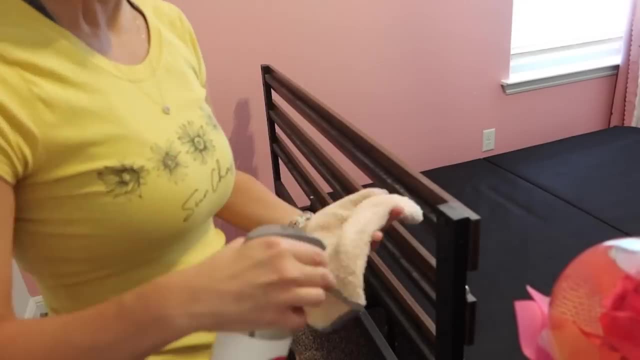 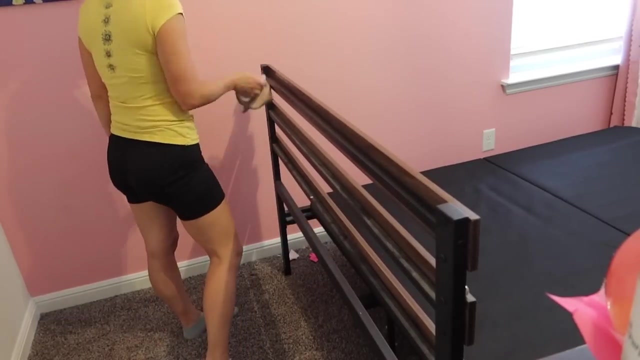 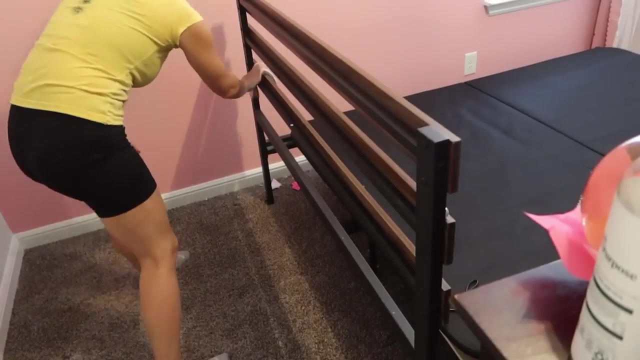 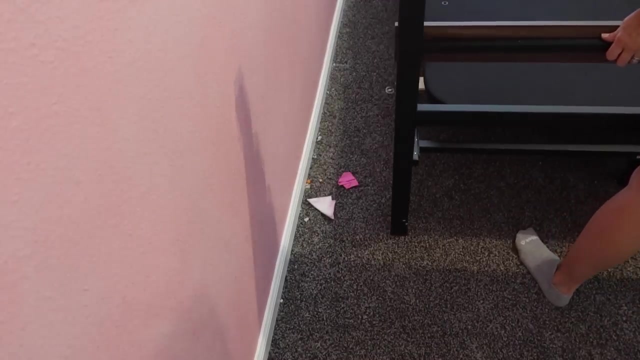 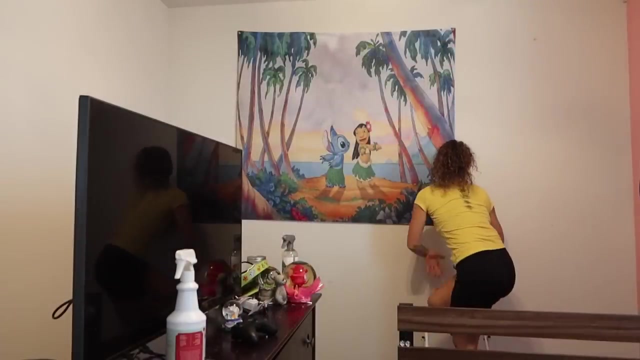 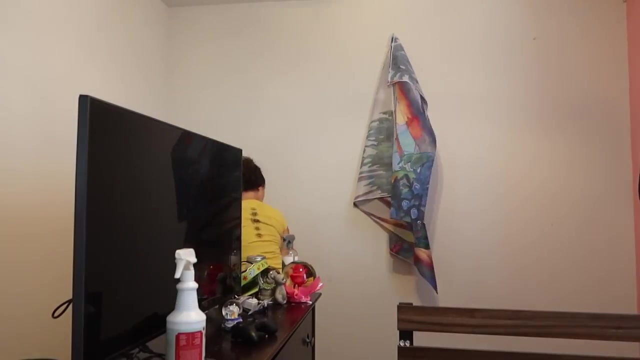 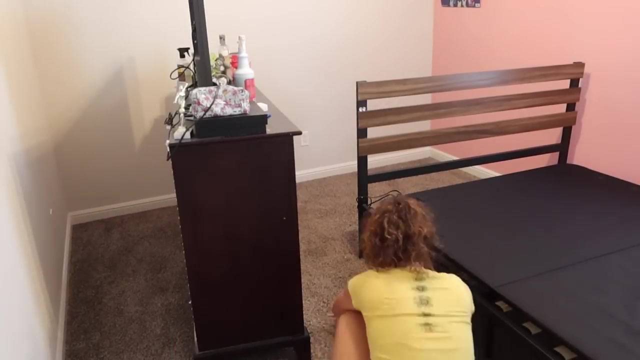 it just gives a new feel to the space and a good revamp. when I'm with you, stars and your body got my eyes and your body got my eyes and your body got my eyes. if you guys been here for a while, then you are not shocked by me, for 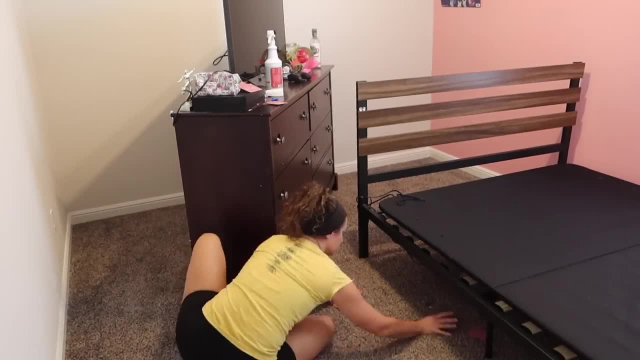 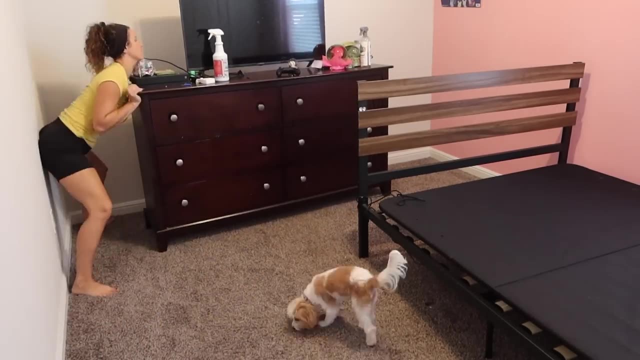 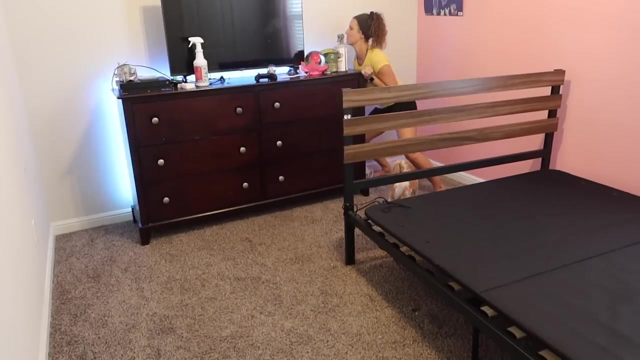 moving my furniture with my feet, because I am a huge like independent, do-it-myself type of person and I don't like asking for help. so I knew I was going to find a way to move the dresser, and using your legs is a great way. if you guys can't move something, try using your legs usually. 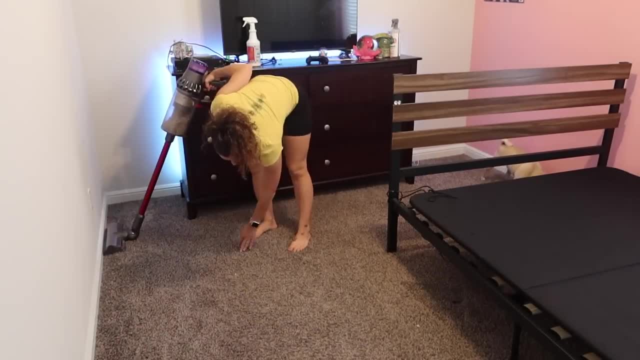 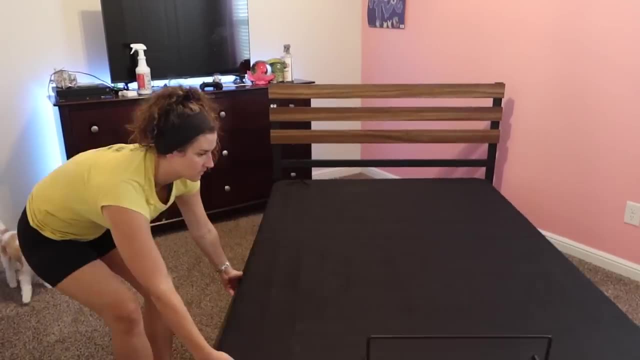 I have to have a wall behind me, and I have to have a wall behind me and I have to have a wall behind me so I can, like, use my arm and push off of the wall with my legs. so definitely give it a try if you are like me and you're stubborn and you don't like to wait for people to help you. 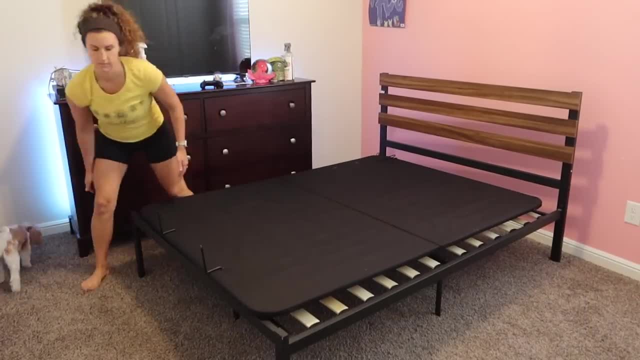 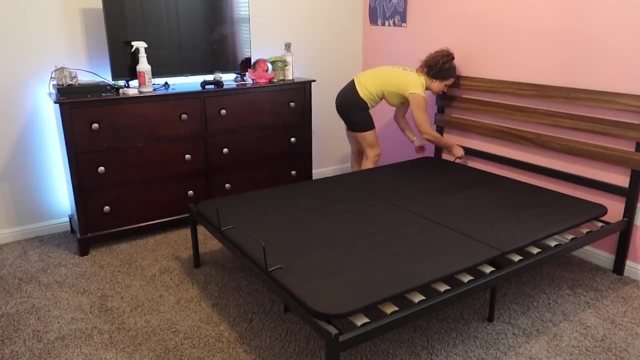 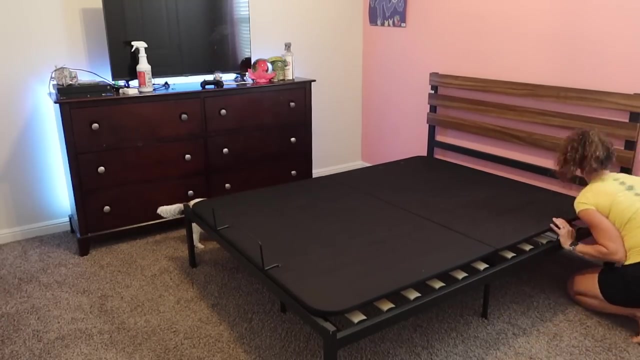 it's a great way to move stuff, but got the dresser moved over, now it's time to get the bed in place. I was hoping to put it a little bit closer to the window, but because of that outlet right there and I needed to plug in Adrienne's adjustable bed frame, I had to shift it over just a little bit. 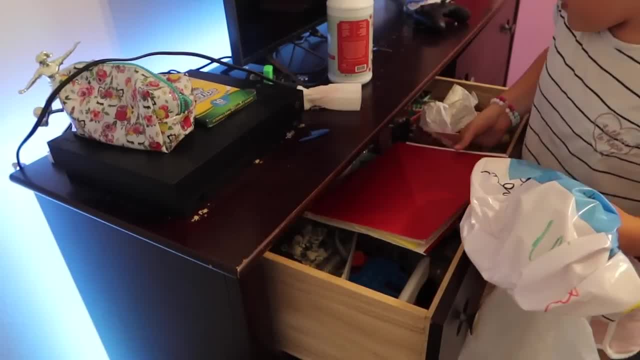 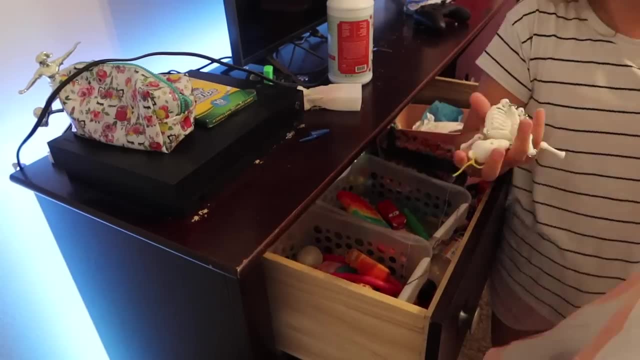 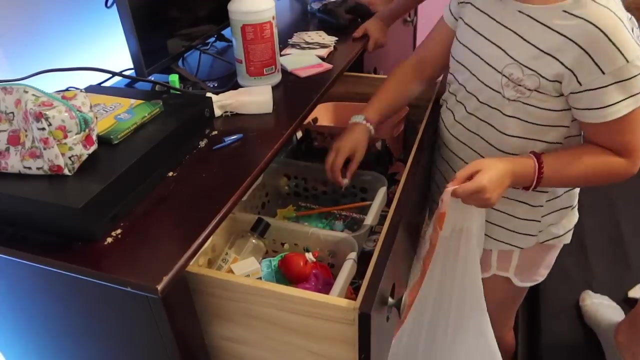 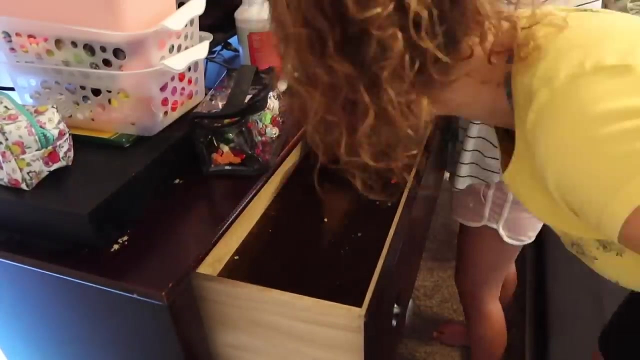 but I really love how this room is looking. it's so much more open feeling, and now it's time for Adrienne to go through her chores and get all the stuff out of there that she no longer wants. it was really cute, though, as she was cleaning the things out. she was like 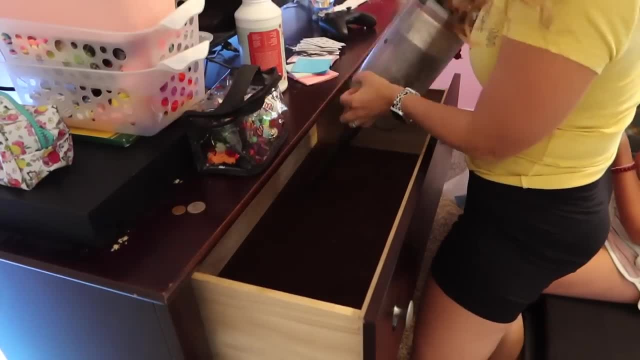 telling me what she was going to do and I was like I want to go through her chores and she was me different stories on different fidgets and when she got them and it was really sweet. but I'm really proud of her. She got rid of a lot of things. 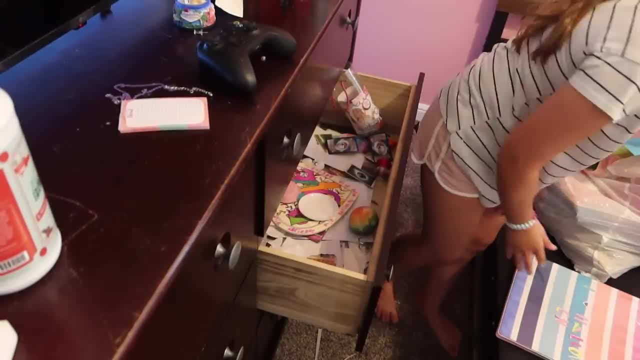 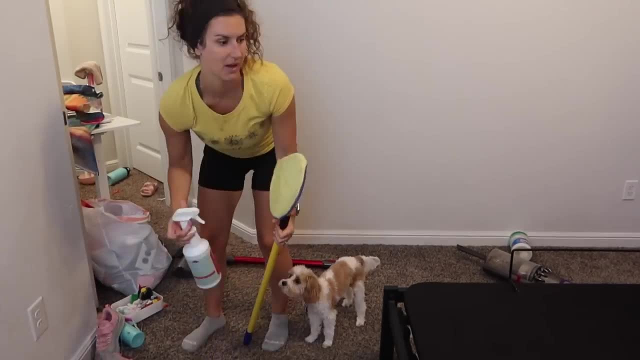 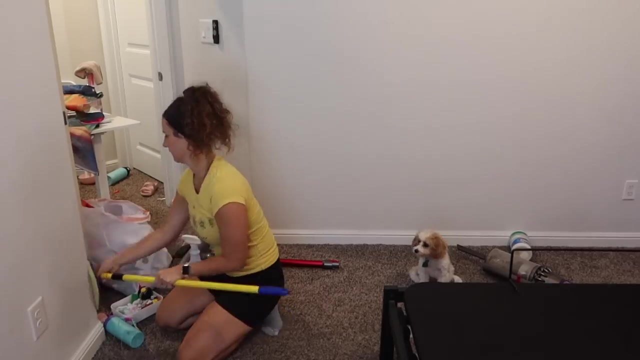 And as she was finishing up in her drawers, I went ahead and started cleaning the rest of the walls in here. As you can see, Stella was so intrigued just watching me clean the walls. She is so stinking cute. In case you guys are wondering, I do get asked a lot what type of dog she is. 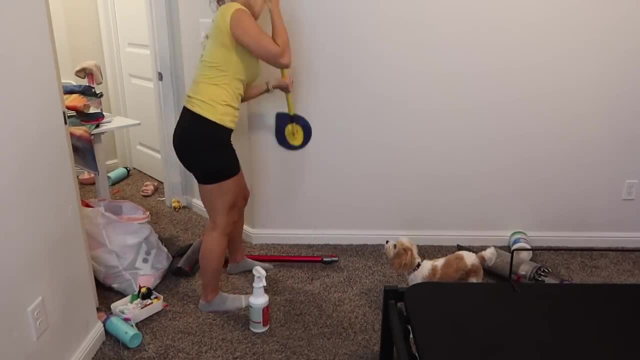 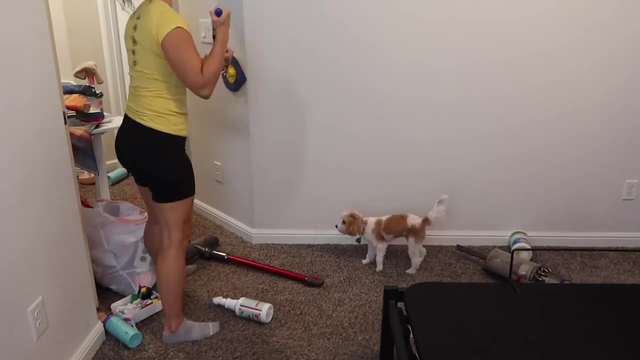 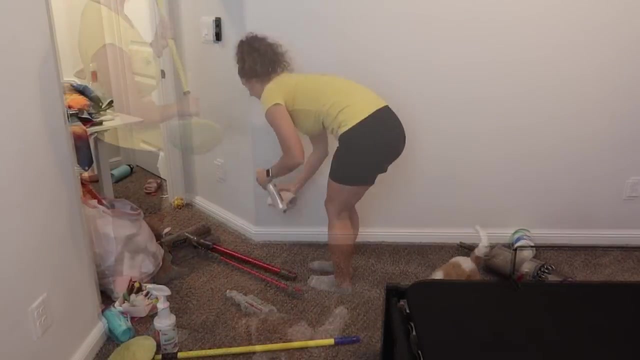 and she is a Cavapoo, And I recently did a Q&A on my channel and I had a few other questions come in and one of them was: when did I get Yoda, Which Yoda is my other dog. He's a pug and we actually got him. it's now been five years. 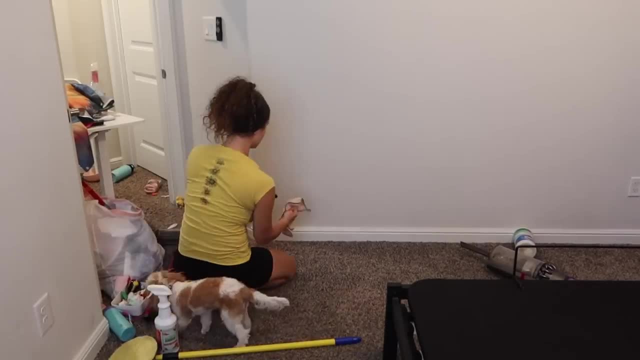 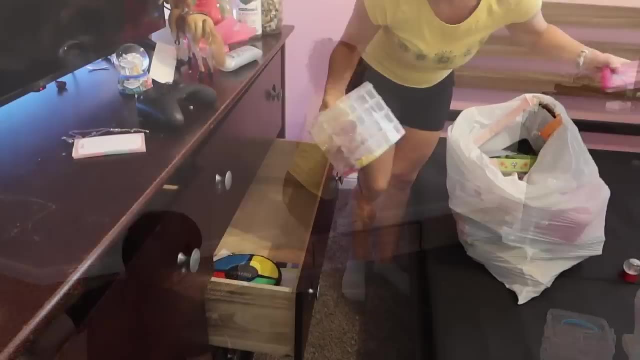 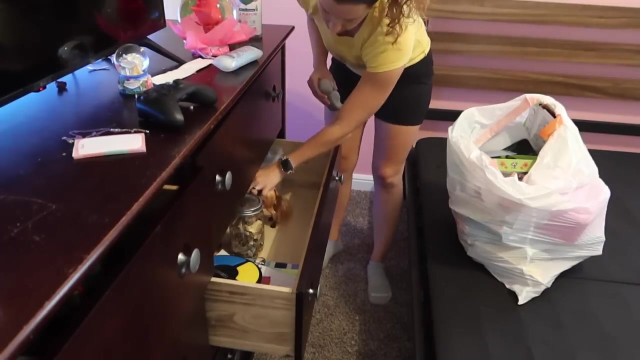 He's- yeah, he's gonna be five years old in November and we got him in San Antonio. We found him off of Craigslist and we were on the hunt for a pug, So that's how we got him. He was actually the runt of the litter, which is always my favorite. I'm a sucker for the runt. 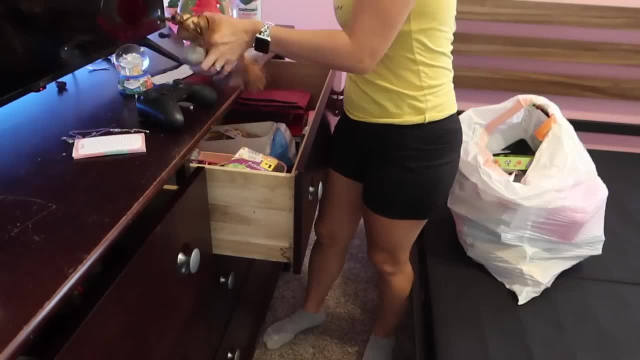 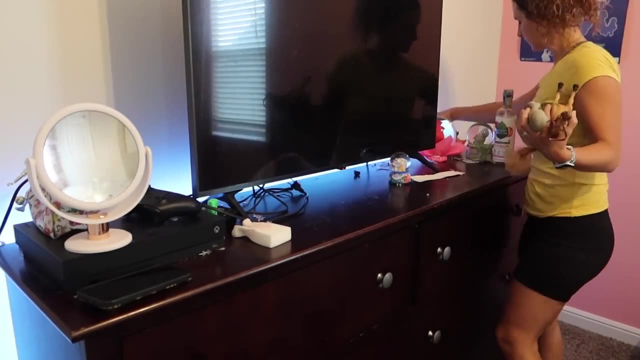 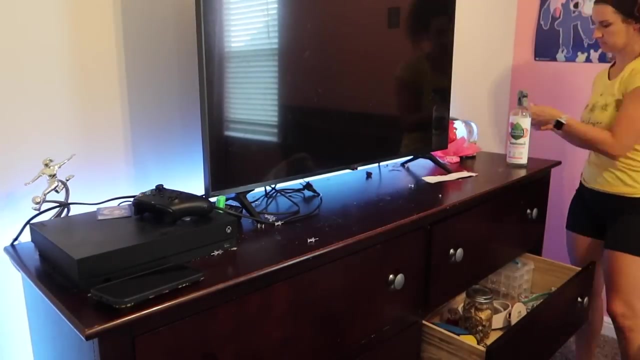 So that is where we got Yoda. Adrian filled up almost a whole bag of junk from out of her dressers. So big progress. Now we were able to organize it inside of little bins and put it back in her dresser nice and neat. That way she. 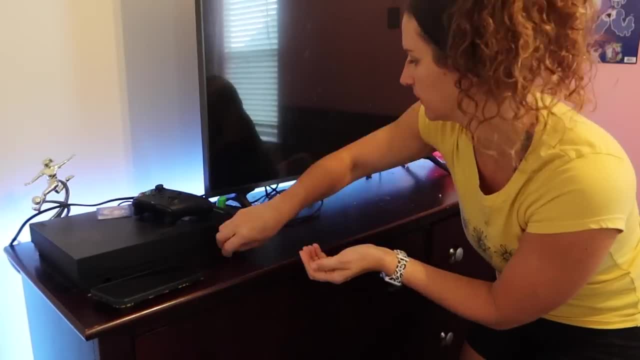 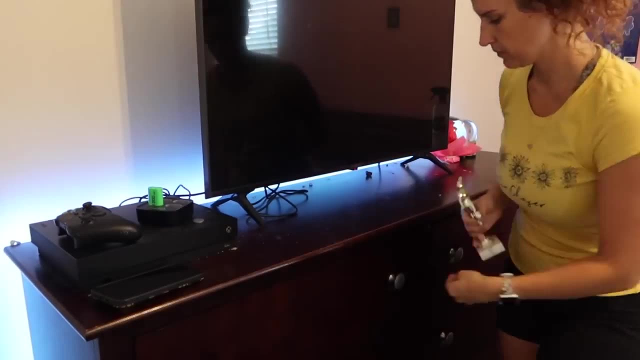 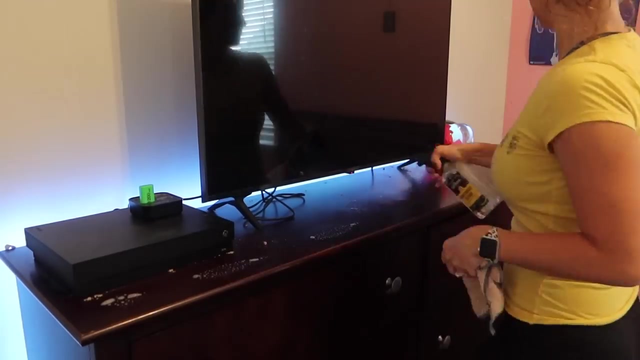 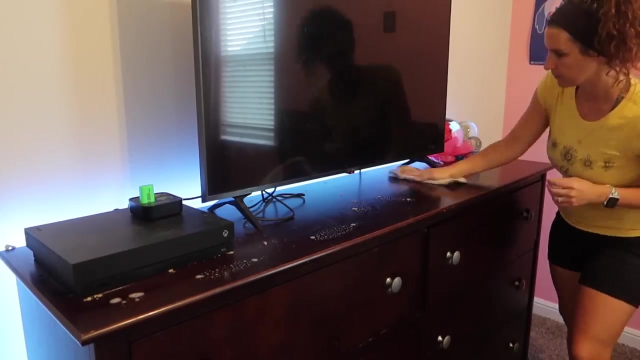 can find whatever she's looking for. So now I can finally clear away the dresser top and wipe it down. But I'm not gonna sell my soul just to be someone you wanna know. Who you like is out of my control. I'm okay being me. 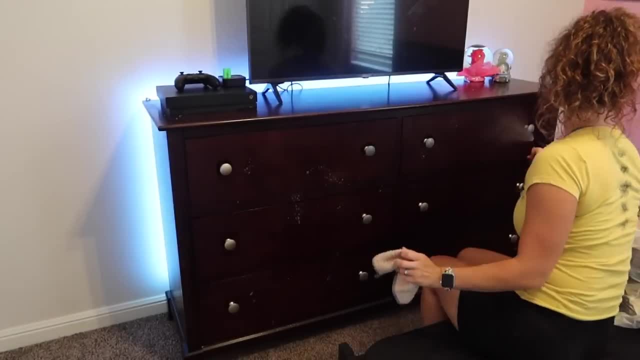 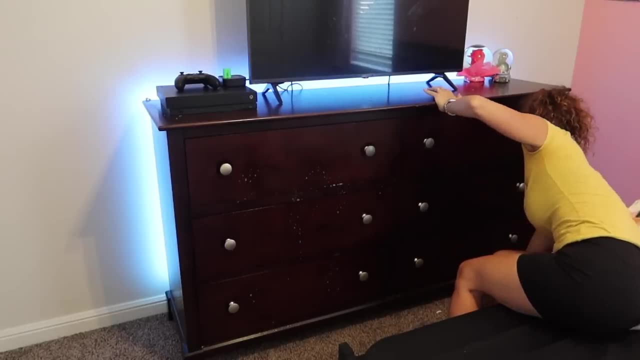 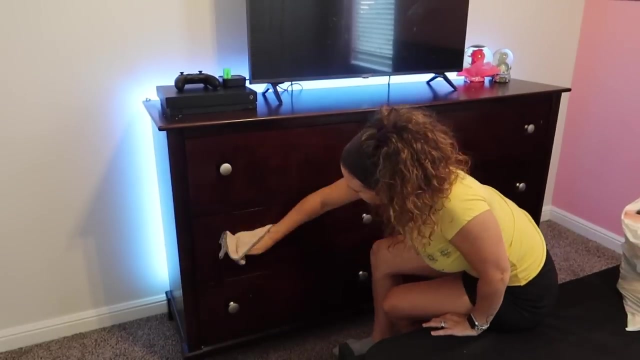 I'm not gonna change myself just to make you fall under some spell. Rather be alone than be a shell. I'm okay being me. You say you don't judge and your friends all agree. They see you fool you, but they don't see what I see. 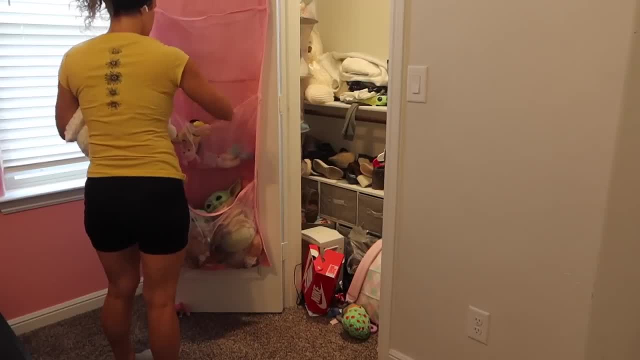 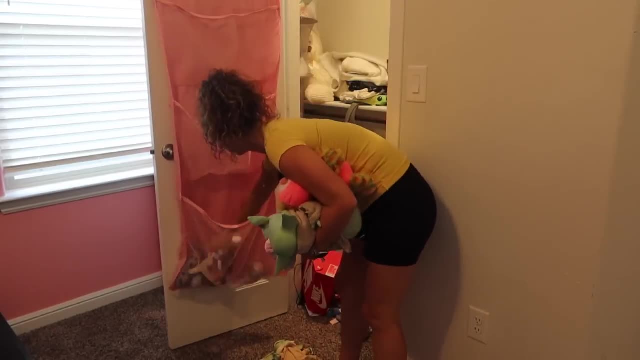 Now it's finally time to tackle this closet. As you can see, it is jam packed with stuff- Mainly stuffed animals and clothes- on the floor. but what I'm going to do is I'm going to pull out all of the stuffed animals that are in the organizer Go put them into the game room. 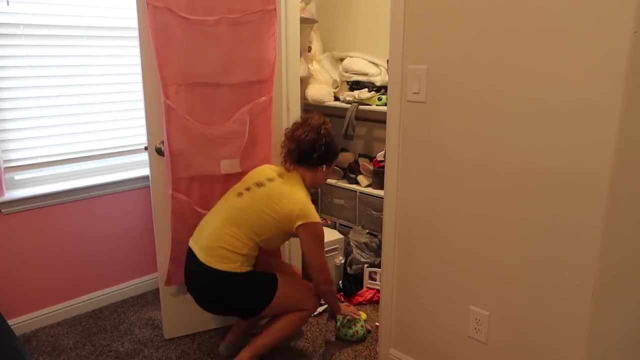 That is where Adrian's at and she's sorting through them, seeing which ones she wants to get rid of. So I went ahead put all the stuffed animals a bit in the game room. so if I had- right now- this is something that's really important- to always check the closet. 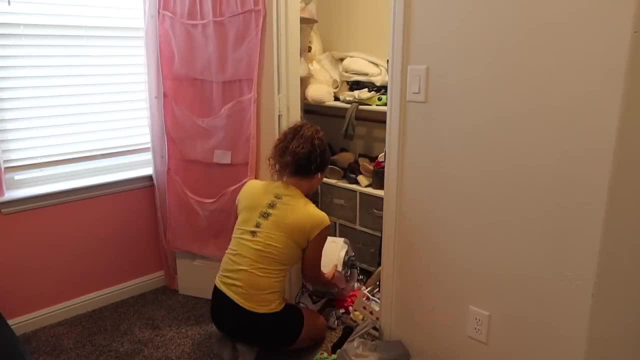 So I went ahead, put all the stuffed animals a bit in the game room. so if I had left full, also I hadあー's basket and whatever she likes. put all the stuffed animals over there, and now we're gonna go through her drawers. she also had. 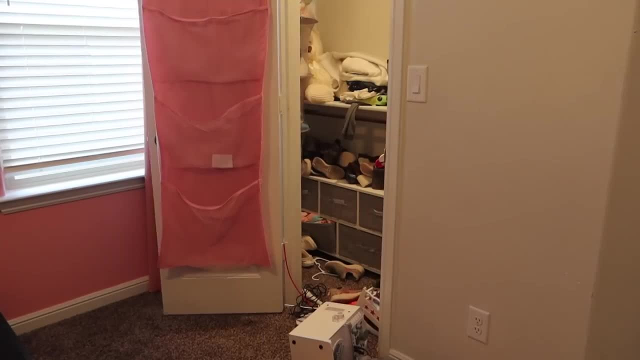 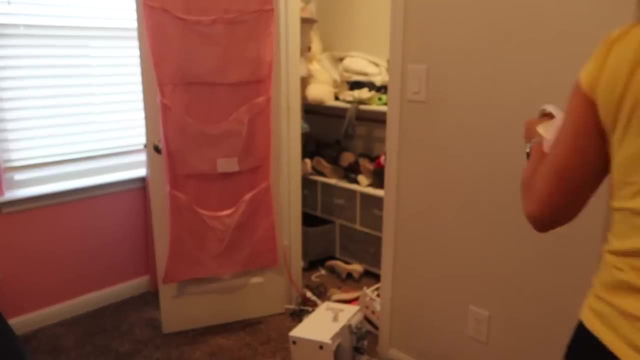 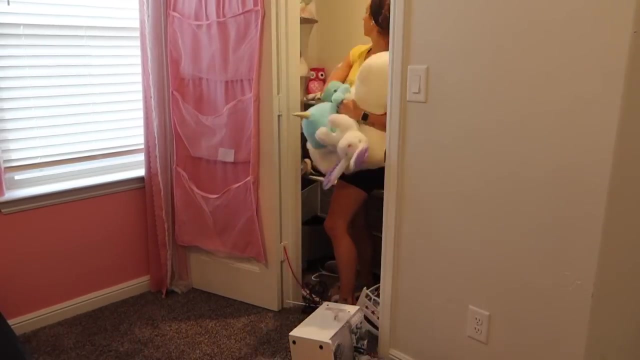 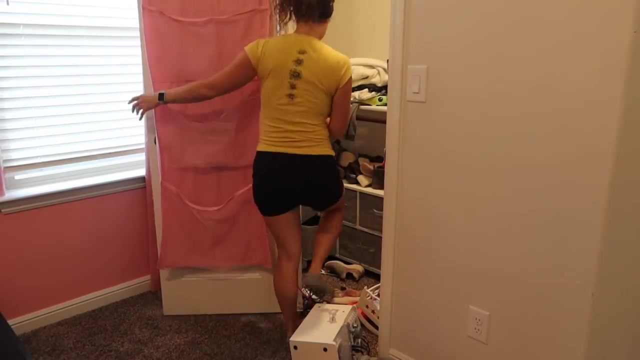 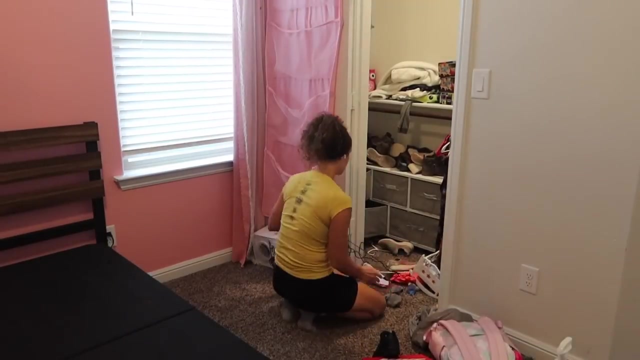 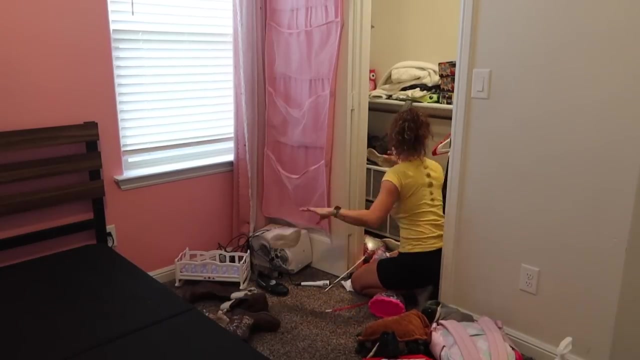 more stuffed animals inside of those. I wanted to go ahead and answer another question that I missed from Claudia, G 3036 and she said: is Ethan three or four and is he going to go to preschool? she said. I asked because I know our youngest kids are about the same age. I'm enjoying my last year having her at home and since he's at 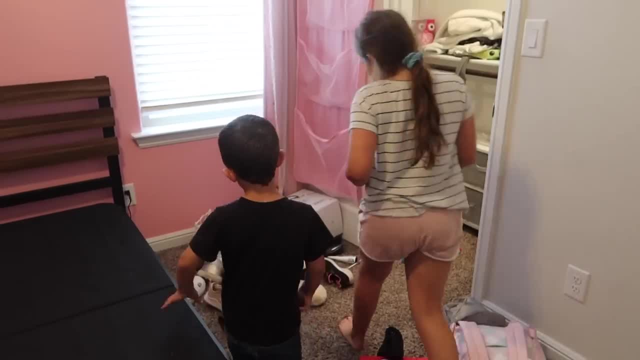 home with me. I was wondering if you want to go to preschool with me, and if you want to go to preschool, you can go to preschool with me. and if you want to go to preschool with me and if you want to go to preschool, we're just going to keep him home until kinder. And how do you feel about that? Are you nervous? 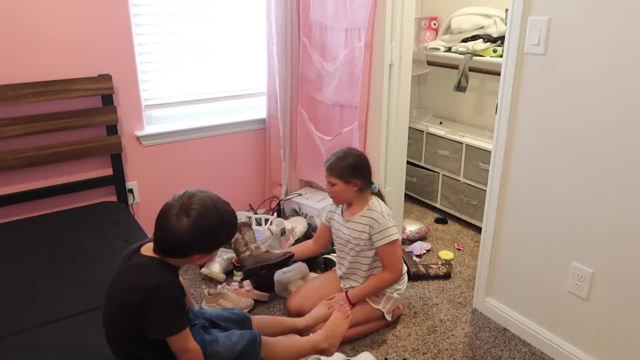 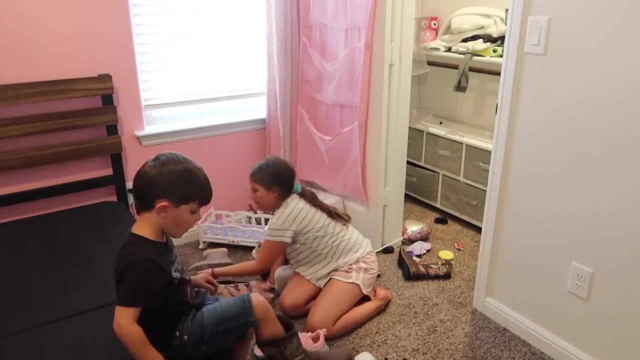 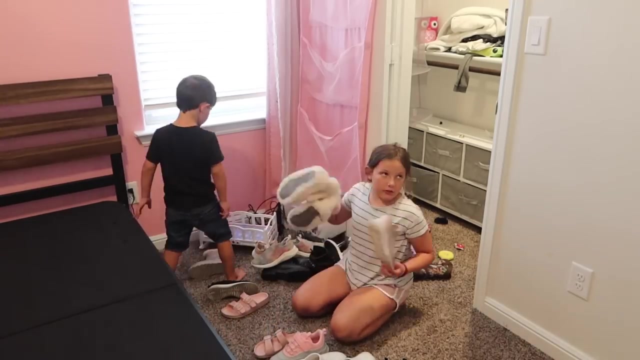 Is he nervous? All of my friends have older kids or they work and their kids have been in daycare, so they can't relate. So Ethan is three and a half. He'll be turning four in October And, because of the way that his birthday falls, he won't actually start kinder until he's almost. 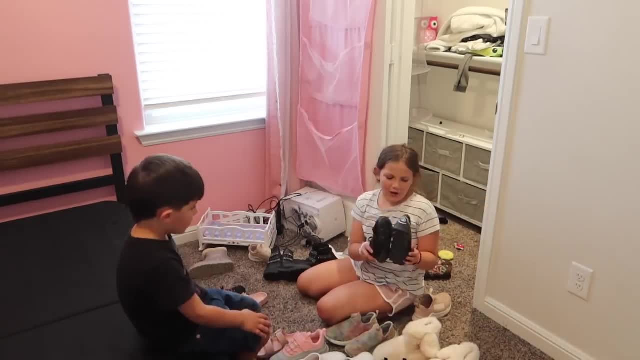 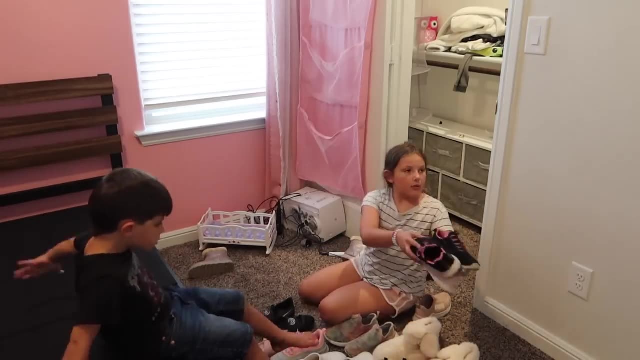 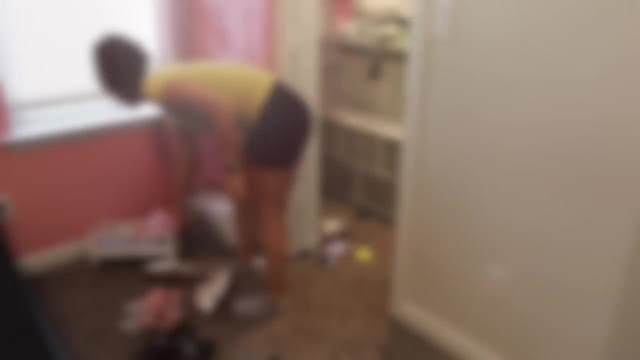 six, And since he's starting late, I am planning on putting him into preschool, not this school year but next school year, because that's when he'll be eligible for preschool. I typically have my kids stay home until kindergarten, but whenever their birthdays, 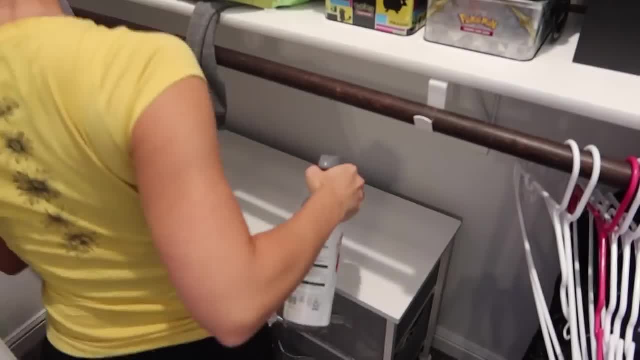 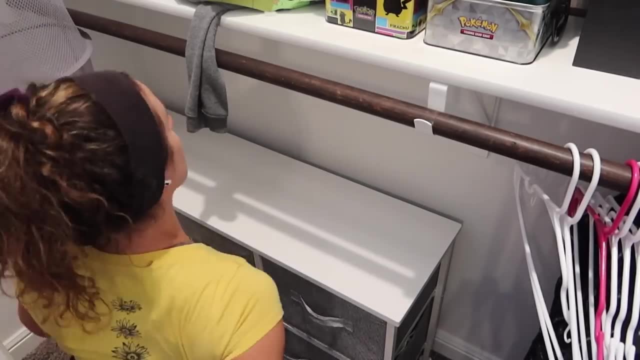 fall like that. I do preschool just because I'm afraid that they might be behind, or what if they're behind and then they're struggling and they're already the older kids In the class? I would hate for them to get held back. So that's kind of my thought process: behind. 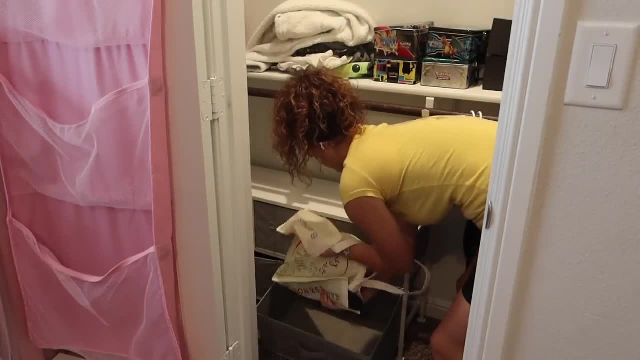 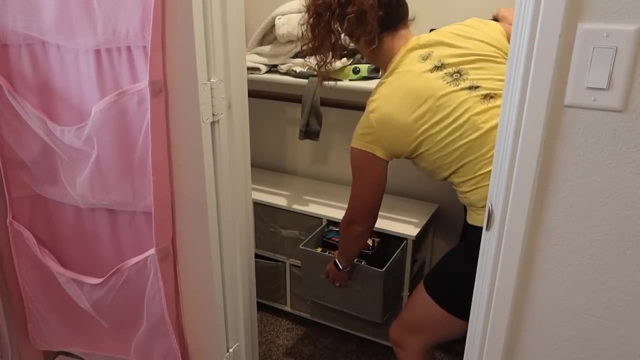 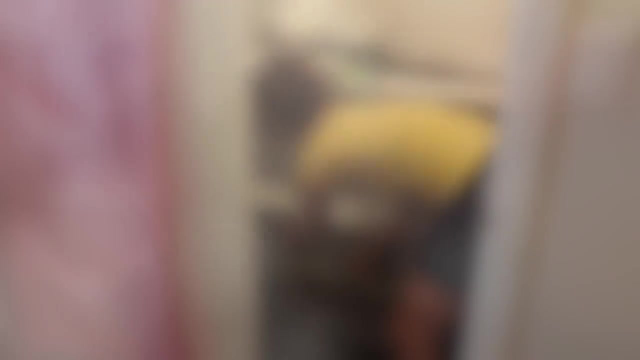 that Adrian is the only other child who did preschool and that's because her birthday fell just like Ethan's. Her birthday is November 1st, So I put her in preschool and I felt like she did really well, She enjoyed it and she was ready, because I feel like she was so close to being 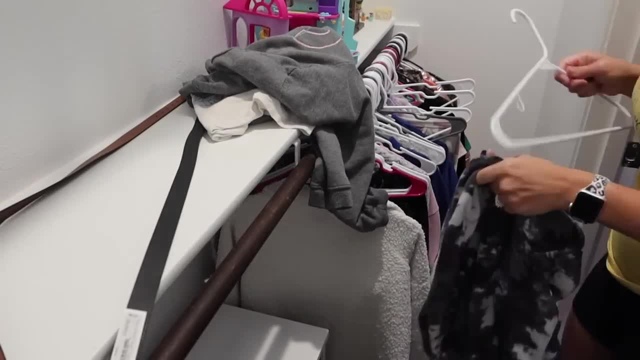 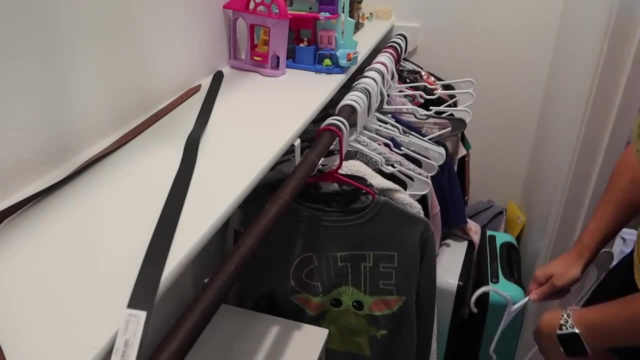 five that she was just ready to start school. So I'm deaf, Definitely nervous about putting him into preschool because he's my last baby And it's just. it makes me really sad because I'm like I know I could keep him home for another year. 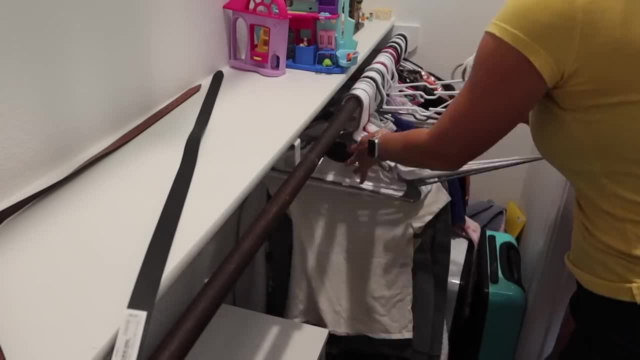 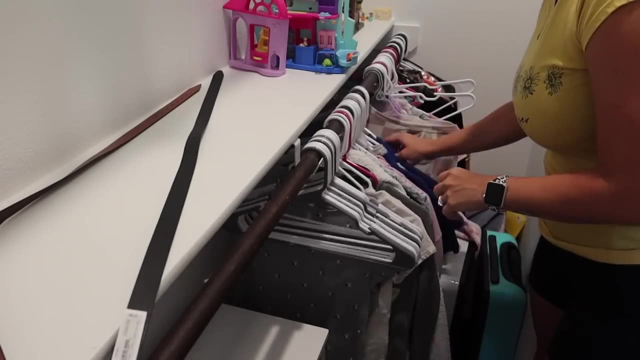 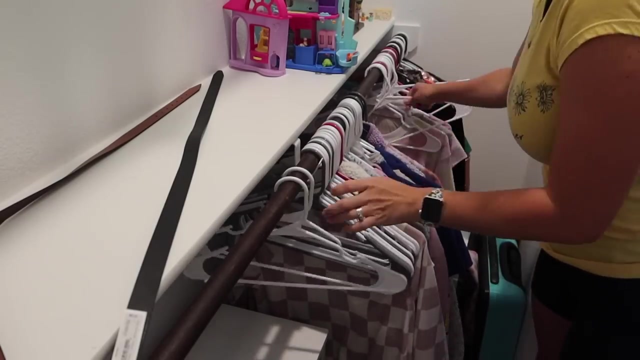 but I feel like he's ready. Honestly, this year I feel like he's ready. He has been asking about school. He wants to go to school every day. He's like mom, let's do our learning book together. So he's very excited about learning and going to school. So it makes me feel better. 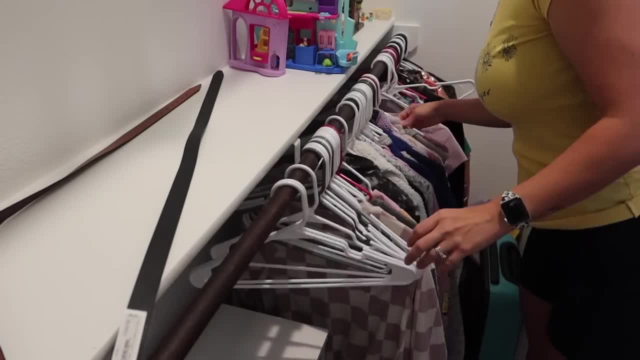 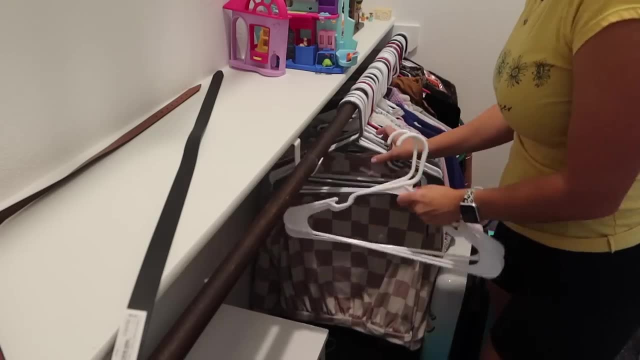 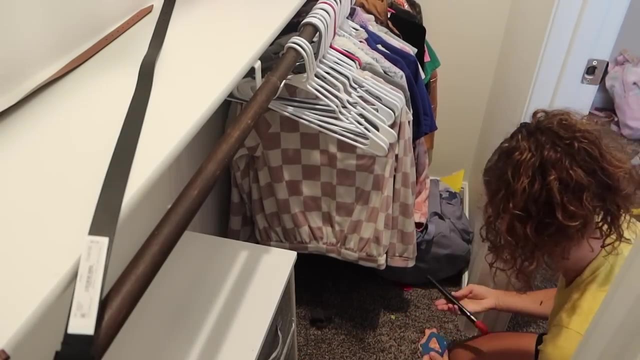 In the decision to put him into preschool. but I definitely can understand, like your feelings of being nervous, because I feel the same, especially because he's my last baby. It makes me just feel really sad about it. But of course I want to do what's best for him And since he's showing a lot, 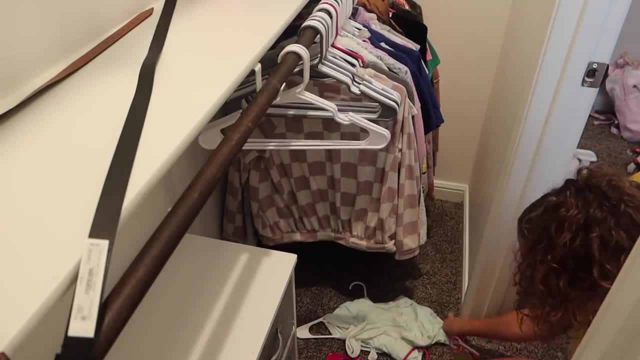 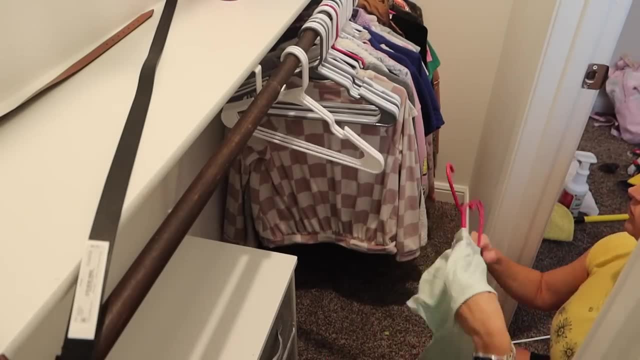 of interest. I do want to do that for him, but I can definitely understand your feelings and why you would keep your daughter at home, And I definitely think you're making the right decision. If that is what your heart is telling you to do, then that's definitely what you should do. Like I said, if Ethan wasn't going to be the older one in his class, then he wouldn't be going to preschool either, Because, honestly, I feel like kids already get so much time in school that I prefer them to stay home, just so they can just spend that extra time at home being a kid. 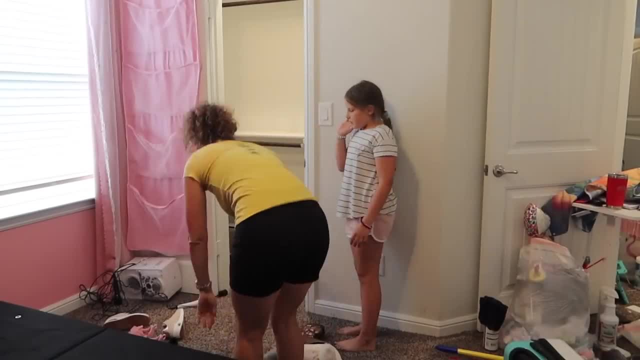 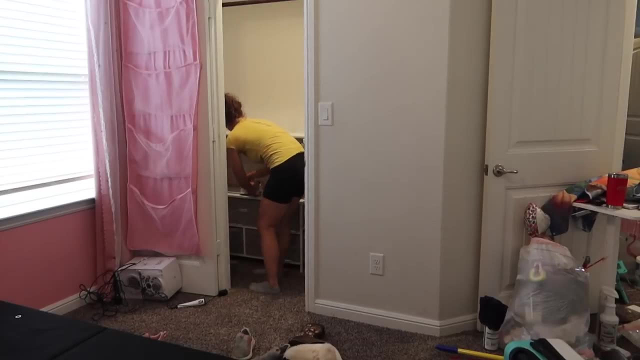 and not stressing about schoolwork and all of that. So I'm all for that. I'm all for keeping the kids home as long as possible, but there's absolutely no shame in putting your kid in daycare. Like I said, you have to do what's best for you and your family. 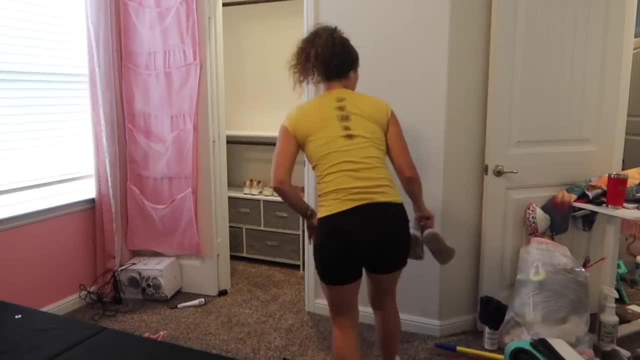 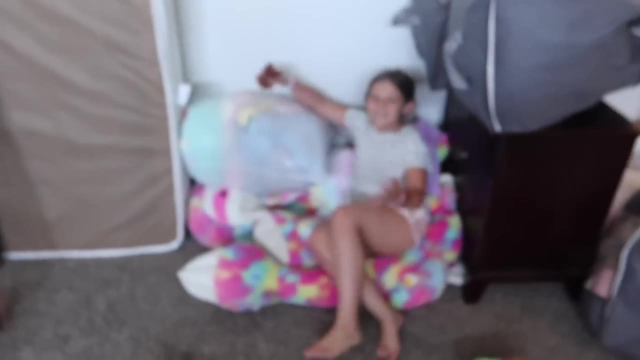 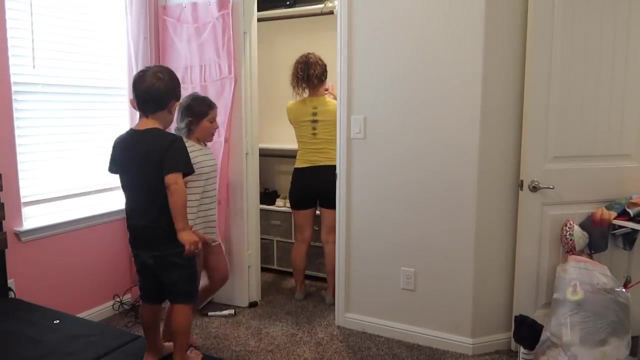 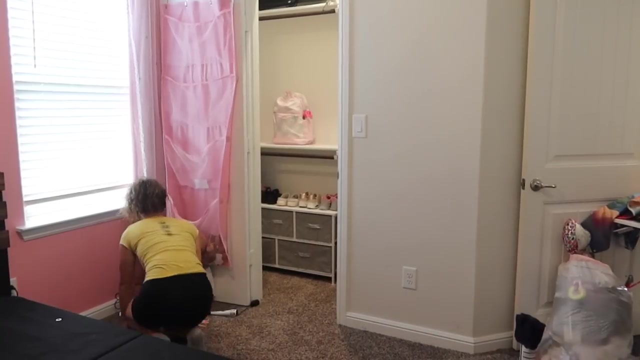 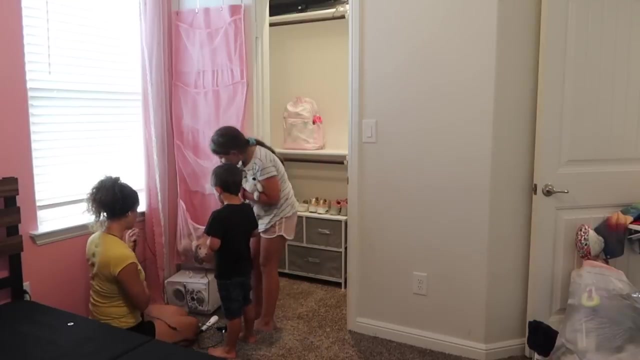 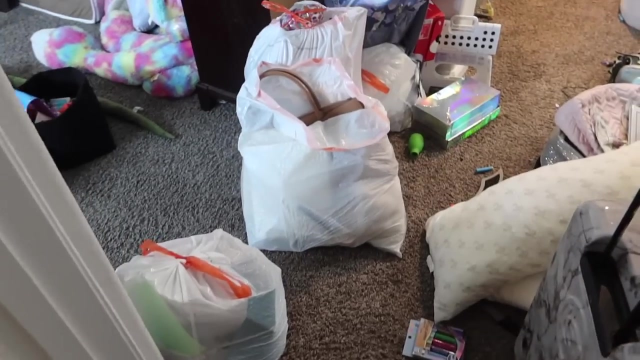 And if you have to work then that's what's best for all of y'all. So Adrian went through all her stuffed animals, got rid of some. there's her pile, So sad. So here is all of the trash. I'm going to see if my husband wants us to hold on to the nightstand. 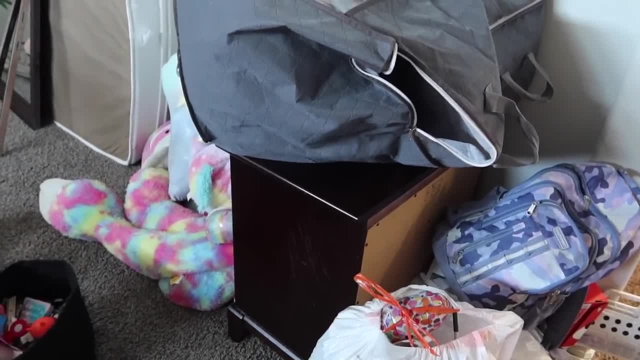 and maybe redo it. We can put it into storage, but I'm going to see if my husband wants us to hold on to the nightstand and maybe redo it. Really love the less cluttered look in her room And she has stuffed animals that she's. 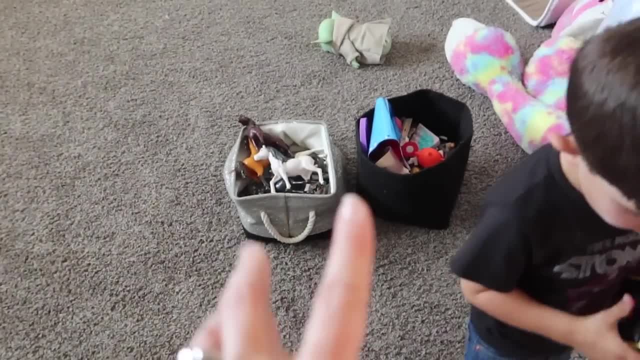 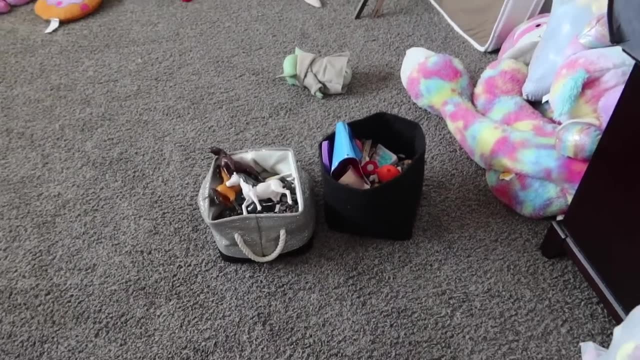 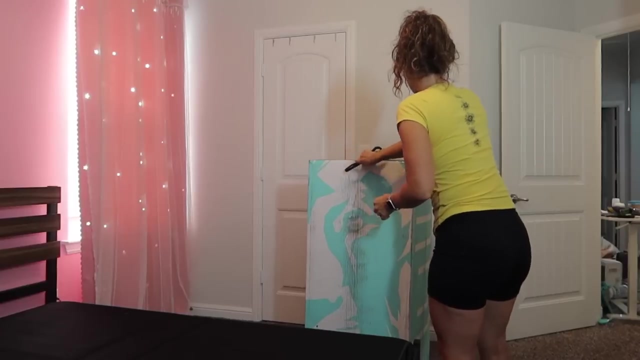 going to get rid of. She's going to go through these last two bins. This is what goes under her bed. Last two little bit of toys. See if there's anything she wants to discard, And then I'll be able to finish up. It's finally time to open up the mattress, The long awaited moment Adrian was. 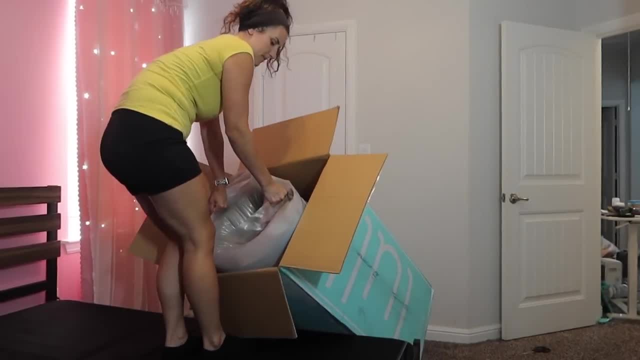 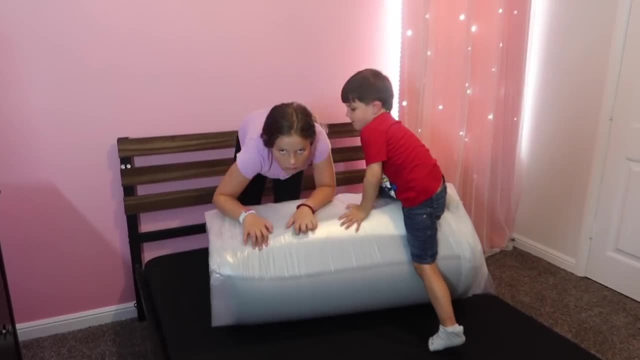 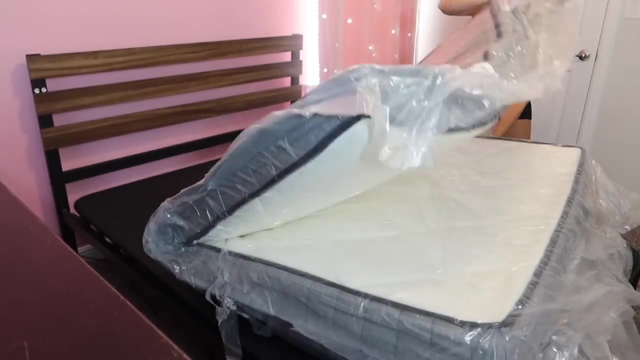 so excited. She could not wait to see it. I'm so excited, I'm so excited, I'm so excited. It took me a little bit longer than I thought to cut through this plastic. I was really scared to hit the mattress, but it was so awesome watching the mattress fluff up. It was really cool to see. 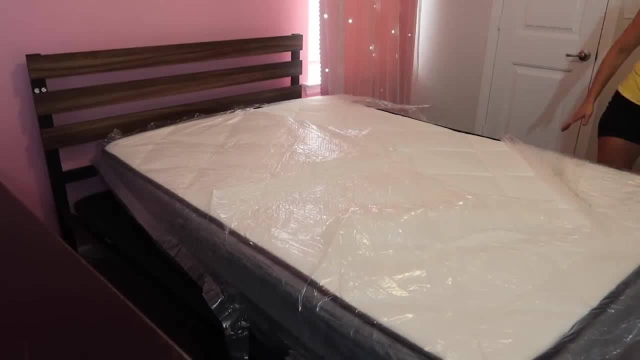 and the kids were so excited to try it out And now that Adrian has been sleeping on it for a few weeks, she is still in love with it. So I'm going to go ahead and open it up And I'm going to go. 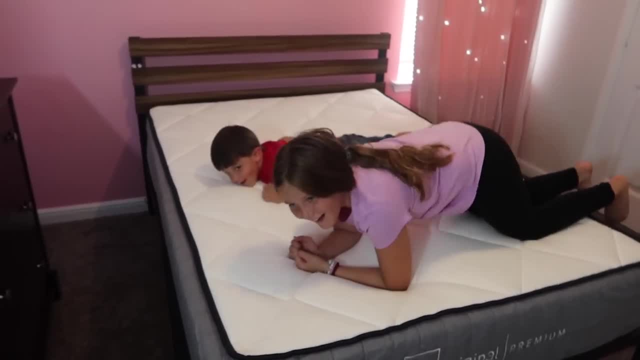 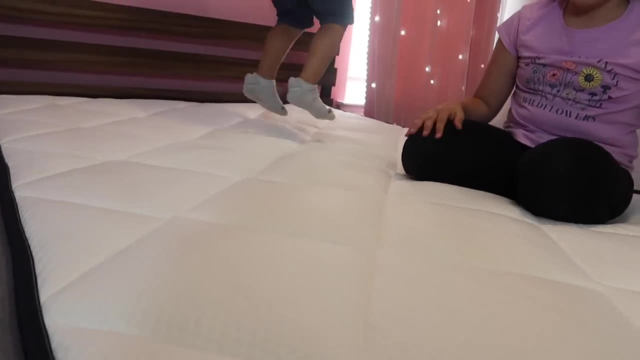 with her mattress and says it is the most comfortable one that she has ever had And it definitely has firmed up. when we first took it out It felt super, super soft. It firmed up some. So if you guys enjoy a little bit firmer mattress, this is definitely the one for you. It is really 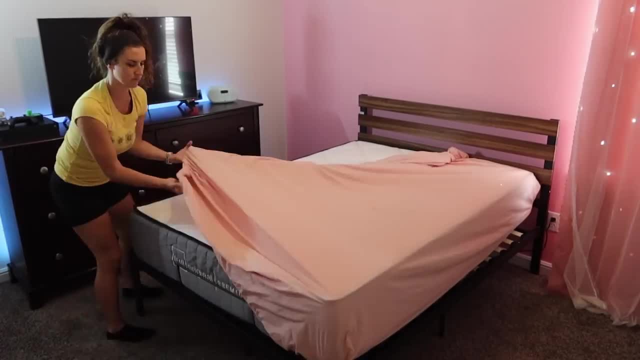 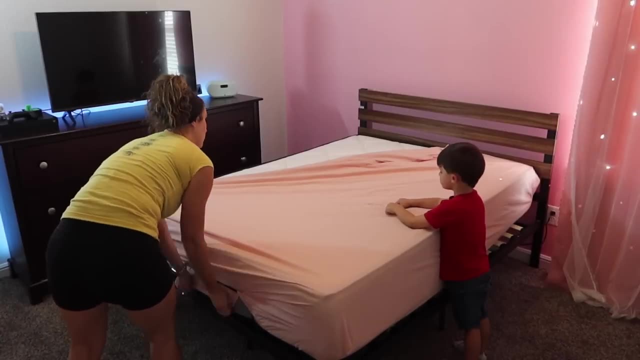 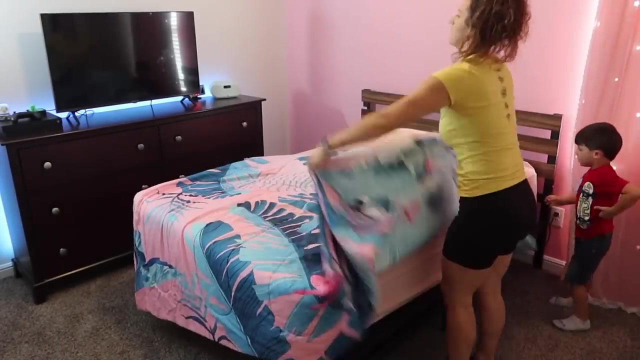 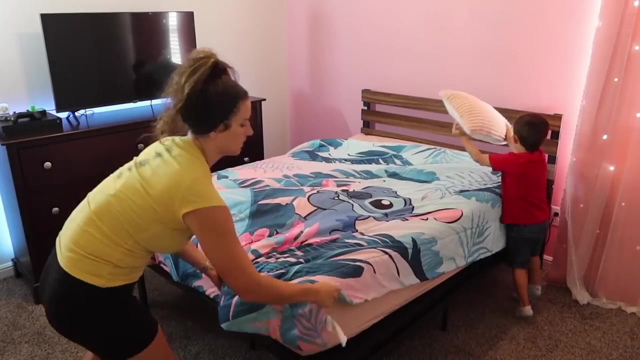 comfortable and great quality. I might be going crazy. I don't know what to do. My heart is screaming for you, baby, And what I'm trying to say is: you make the sky look blue Even when it is gray, baby. 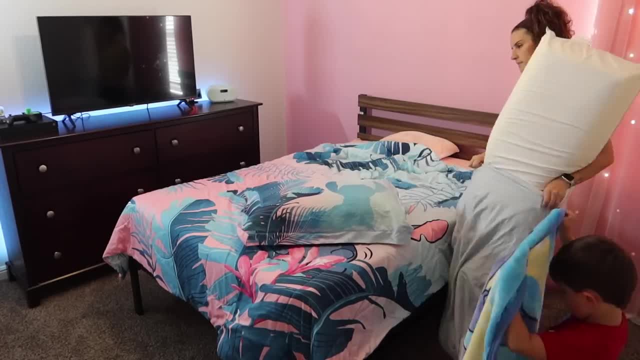 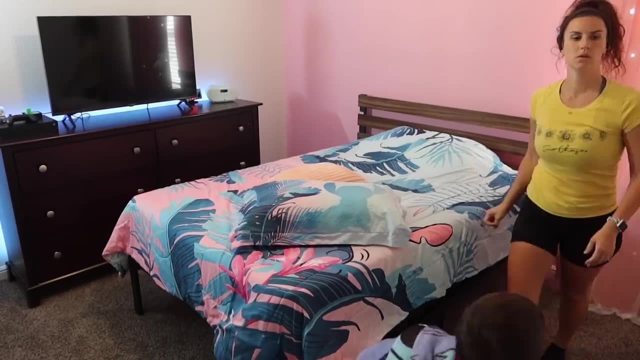 We are putting the final touches on her bedroom. We're making her bed. the sheets and bedding are all fresh and clean. I was planning on hanging the and stitch posters back up in her room, But whenever I got to the part where I was about, 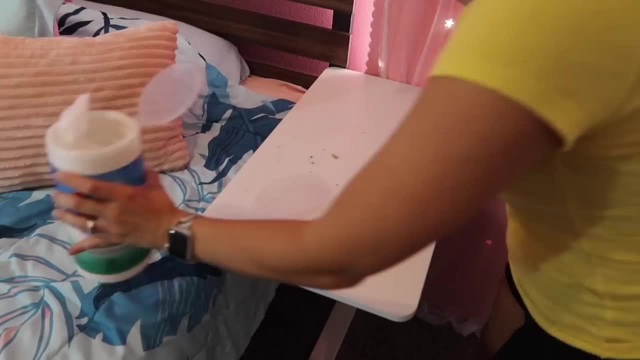 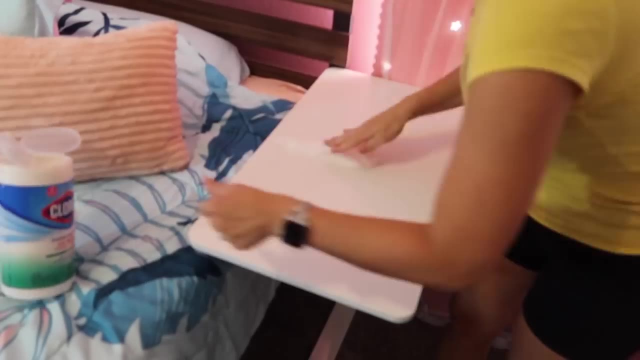 to hang them up. she was like: I actually really liked the way it looks without anything on the walls, So I was like: all right, if you want to leave them off for now, that's fine, I'm still holding onto them. I just I stored them in the closet in case she changes her mind in the future. 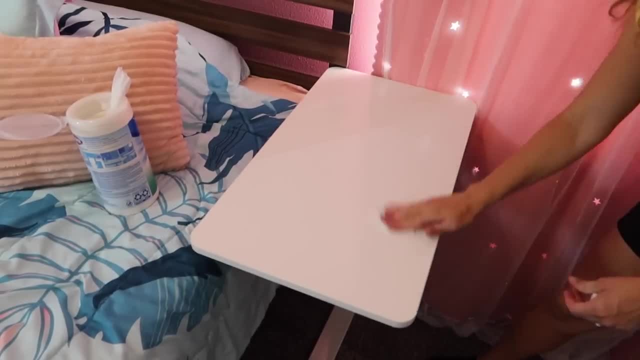 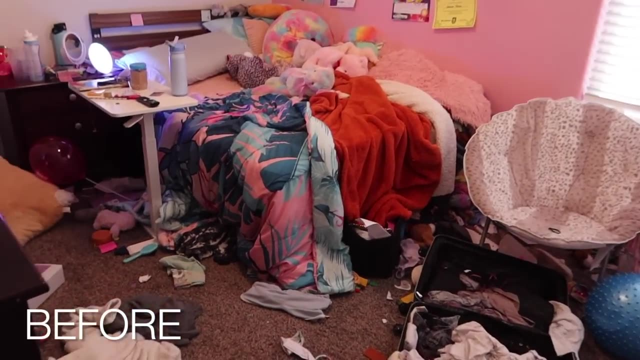 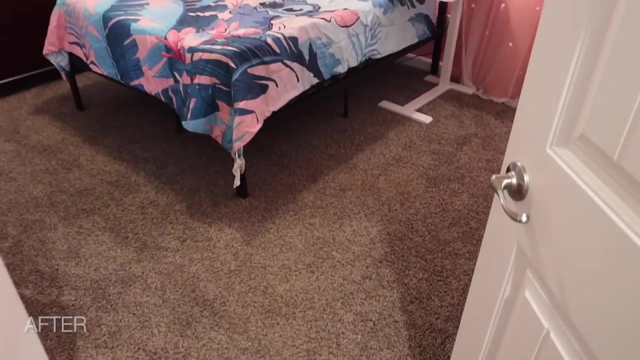 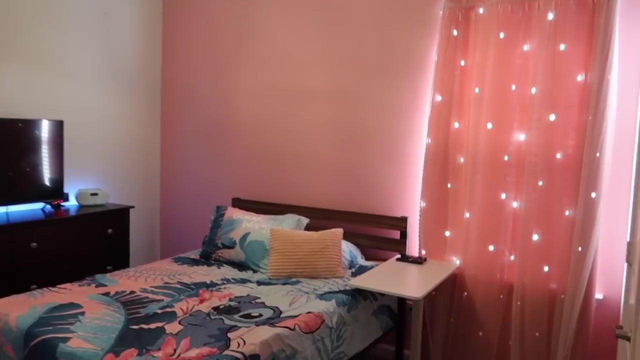 But I love how this room turned out, You guys. it took me- no lie, six hours of cleaning, but look at the after shot. Oh my goodness, I love it. It looks so much better in here- Definitely the most satisfying transformation by far. but I hope you guys enjoyed this video. 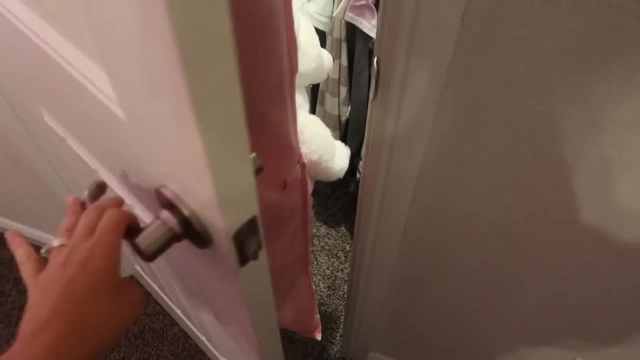 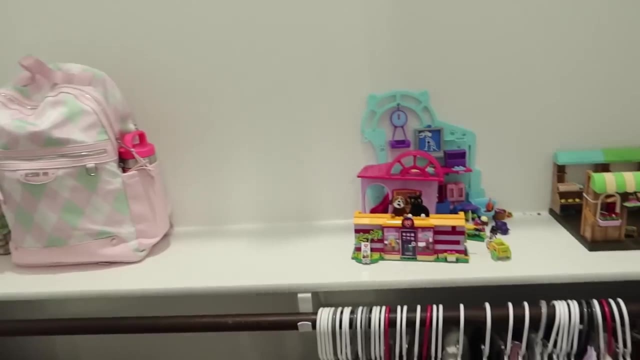 If you did make sure you give it a thumbs up. It really helps out my channel. If you're new and you haven't subscribed, I would love for you to hit that subscribe button. Join my YouTube family. I do upload every single week new cleaning motivation and I would love to have 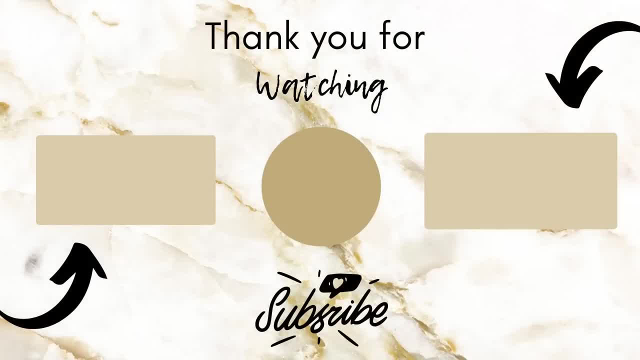 you here, but I hope y'all have a wonderful day and I can't wait to see you in the next one. Bye.